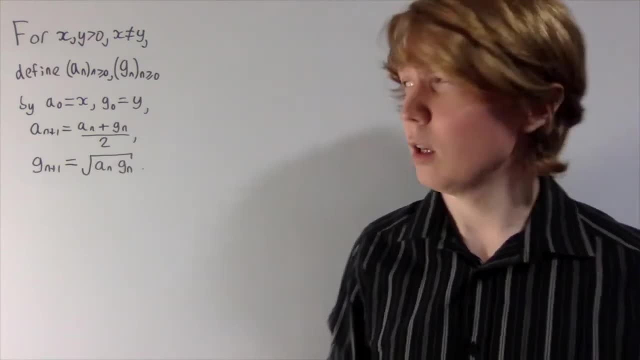 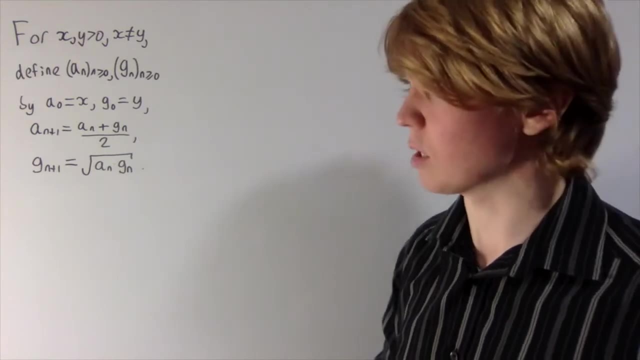 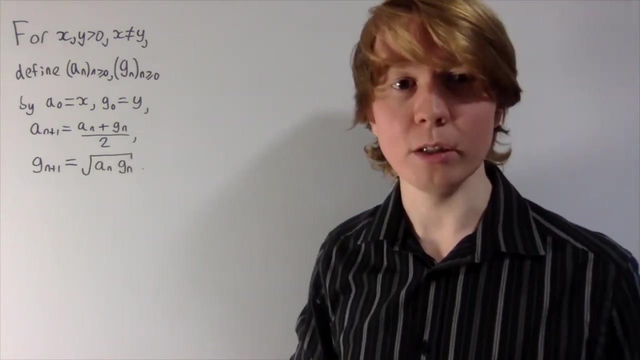 arithmetic mean of the previous term in each sequence And then to find the next term in the g sequence, you find the geometric mean of the previous term in each of the sequences. So for example, a1,, this would be x plus y over 2, the arithmetic mean of x and y, Then g of 1,. 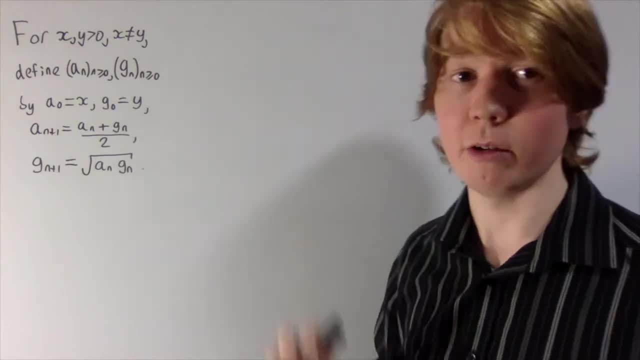 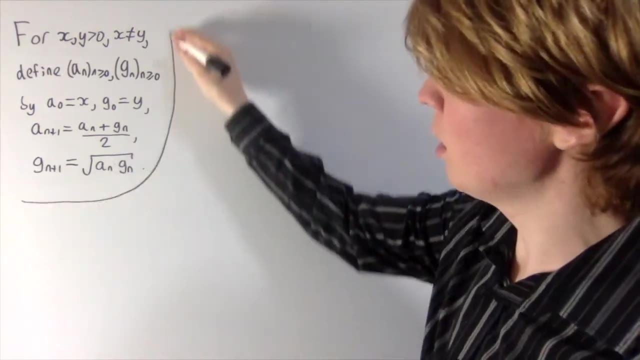 this would be the geometric mean of x and y, so the square root of x multiplied by y. So we're going to be interested in what happens as n goes to infinity for these two sequences. But just before we deal with that limit, we'll have a look at a couple of properties. 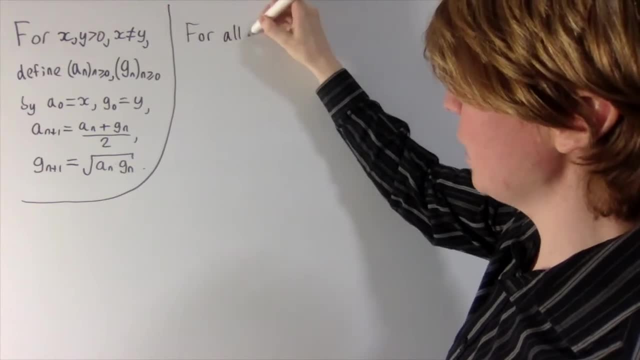 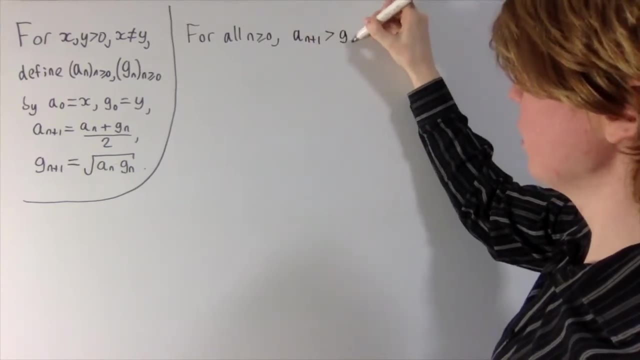 So the first of which we're going to prove is that, for all n greater than or equal to 0, a of n is equal to 0.. a of n plus 1 is strictly greater than g of n plus 1.. So you'll note, here we're starting with a1. 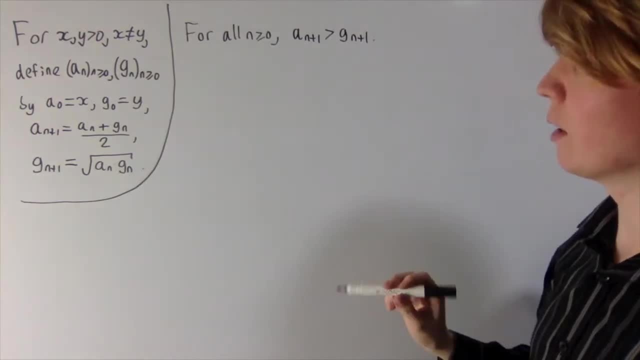 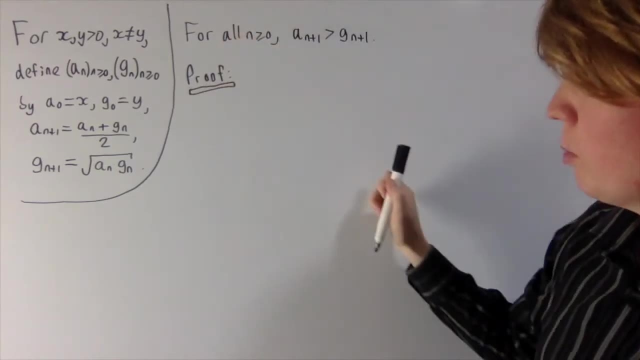 and g1, because we don't know if x is bigger than y. Okay, let's prove this. So how we're going to approach this is: we can look at what is a n plus 1,. this is a n plus g, n over. 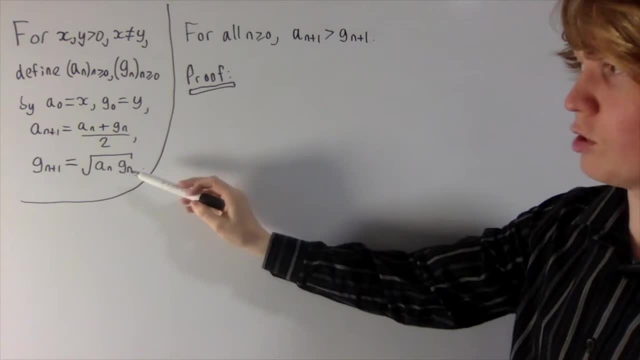 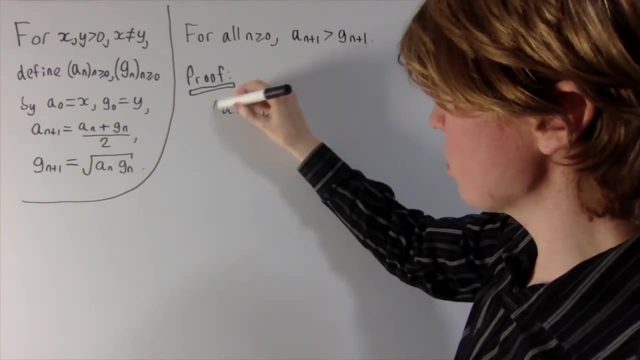 2. What is g of n plus 1?? This is the square root of a, n, g, n. I'm going to begin just by writing a, n plus g, n, all squared. Then I'm going to do some algebra, rewrite this, get an inequality. 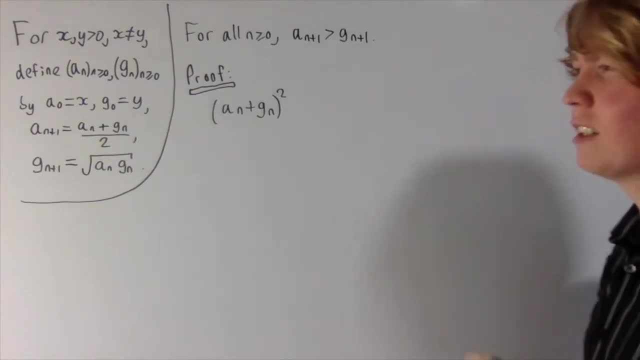 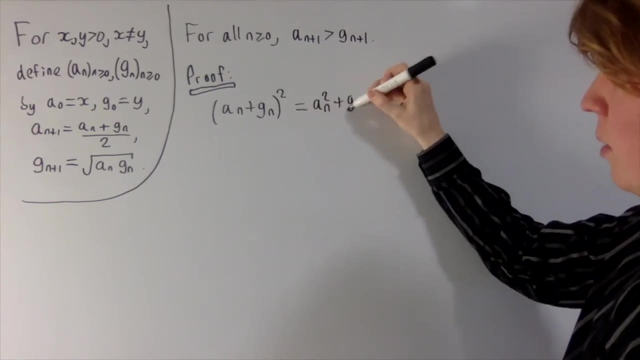 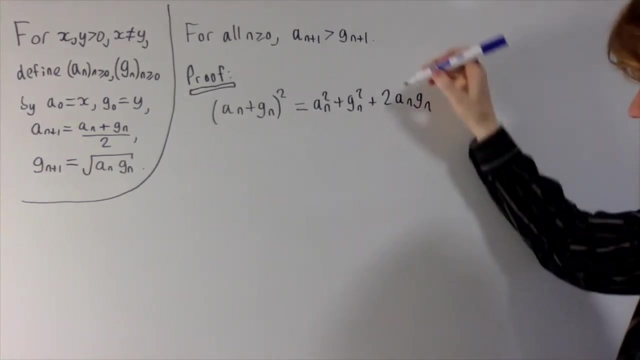 and then I'll be able to show, rearranging this, that a? n plus 1 is indeed greater than g n plus 1.. The first thing I'm going to do is just expand this So a? n squared plus g n squared plus 2 a n- g- n. And then the next step I'm going to use is a bit of a trick here. 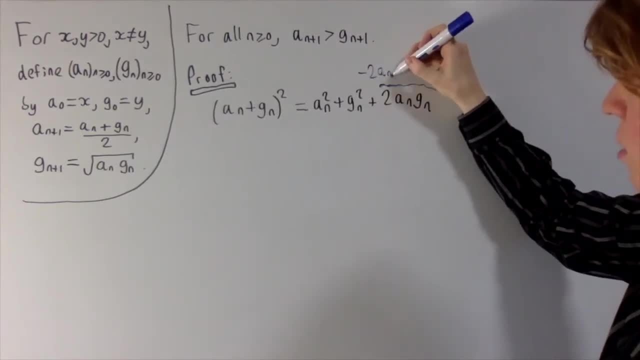 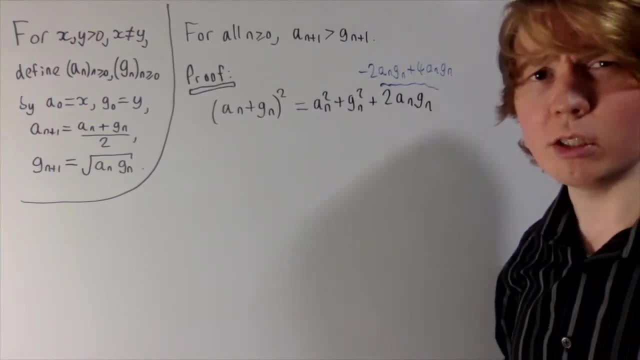 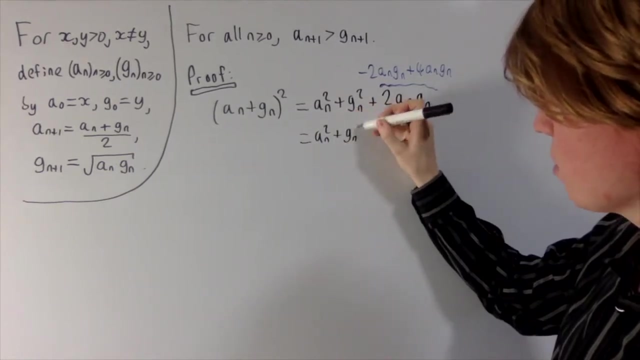 I'm going to rewrite 2 a n g n as minus 2 a n g n plus 4 a n g n. So why on earth am I doing this? It'll become clear in the next step. If I write this out, then as a n squared plus g n squared. 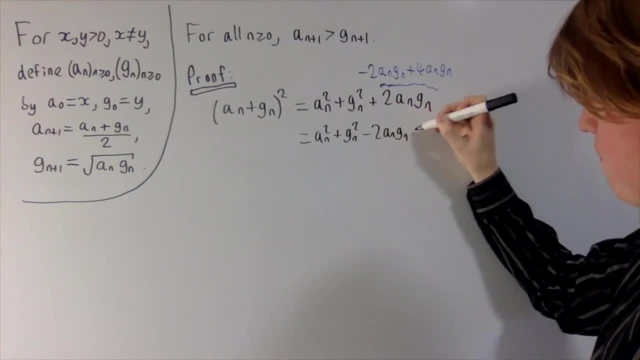 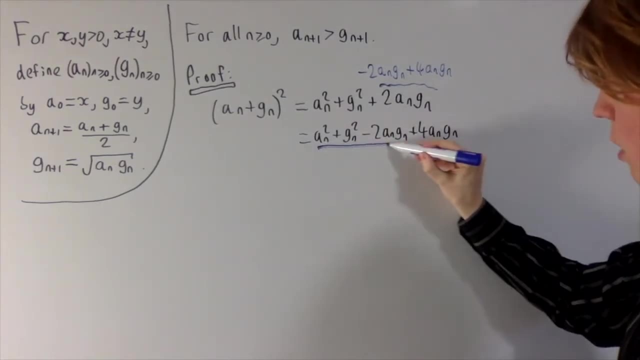 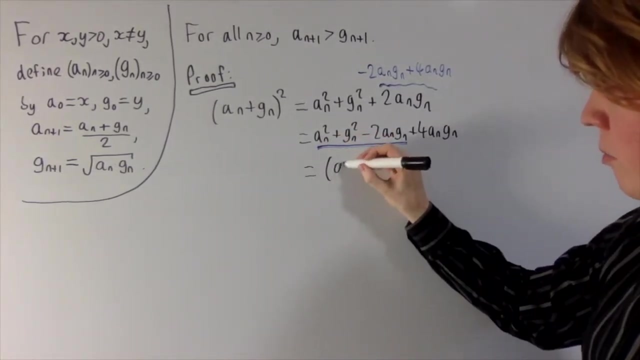 minus 2 a n g n plus 4 a n g n. Well, this thing here now: a n squared plus g n squared minus 2 a n g n. all this is is the square of the difference between a n and g n. So a n minus g n. 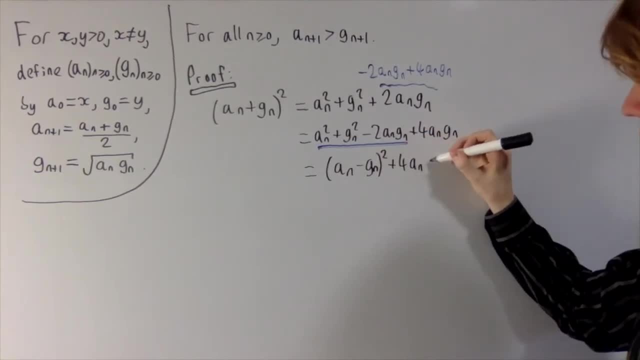 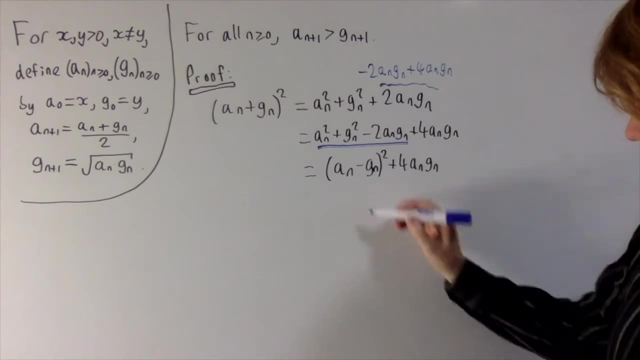 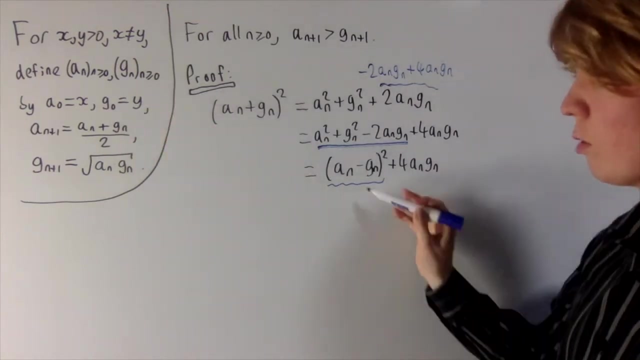 all squared And we've still got this plus 4: a, n, g, n. Okay, so what we need to do next then is, you'll notice, for example, with a 0 and g 0, these are x and y, these are distinct. so 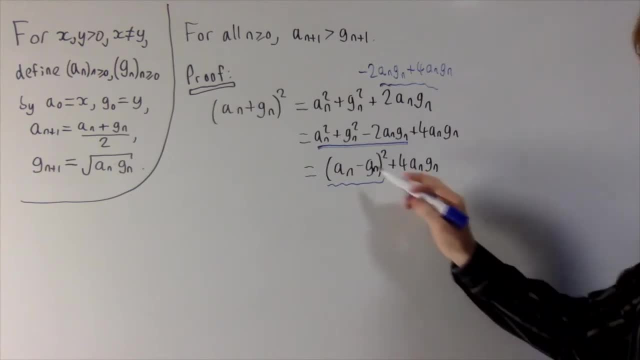 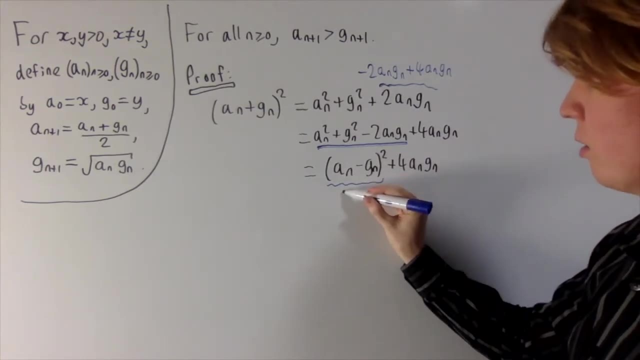 a 0 minus g 0, squared, this is always going to be strictly greater than 0.. And similarly you can show that actually, for every single term, a, n and g n aren't going to be equal if you start with distinct numbers- x and y. So this is why we specify that x is not equal. 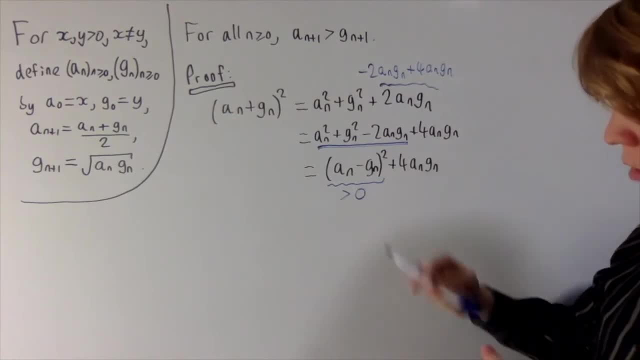 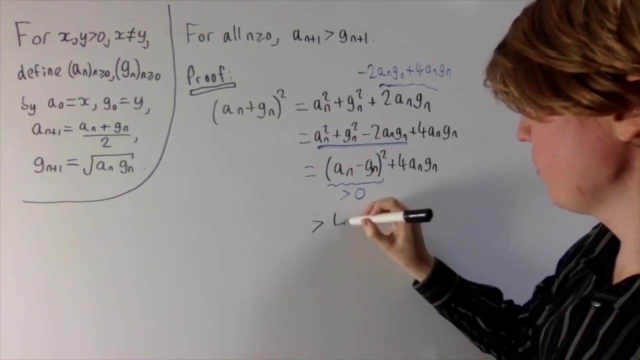 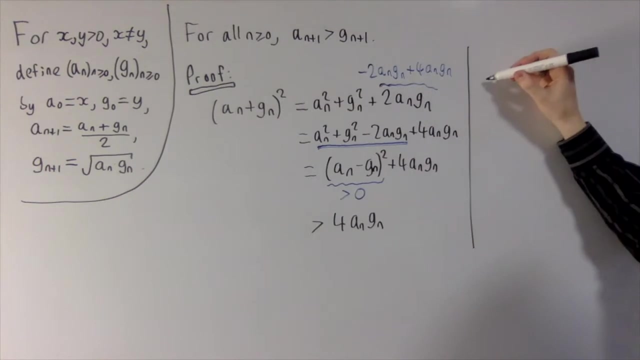 to y there. So this is strictly greater than 0, which means, then, that a? n plus g? n, all squared, is strictly greater than 4 a n. Okay, so what have we shown here? We have shown that a? n plus g? n, all squared, is strictly. 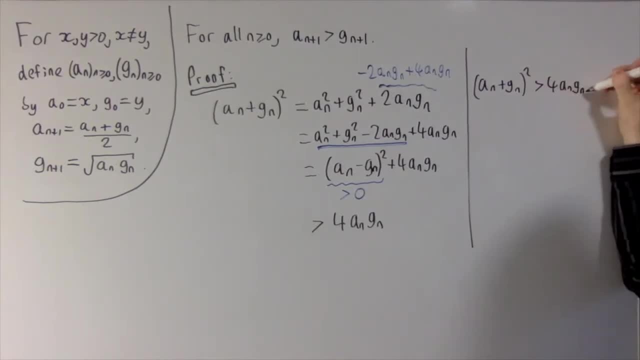 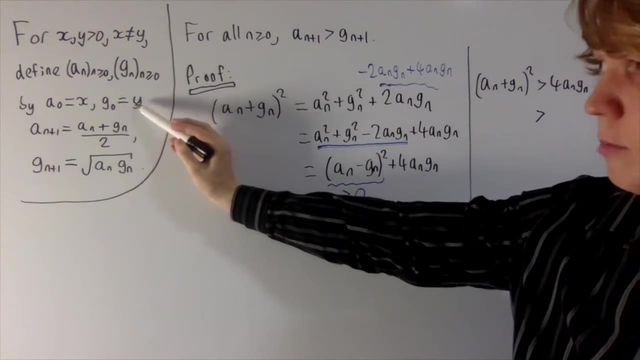 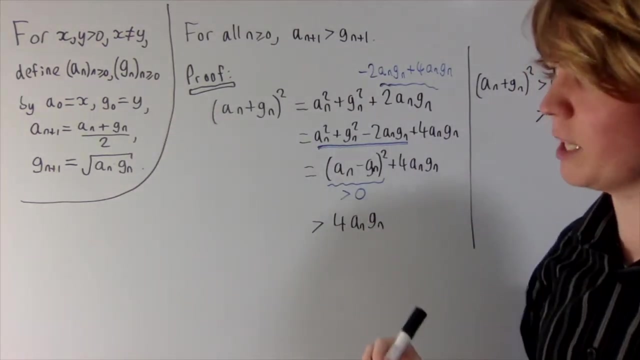 greater than 4: a, n, g, n. So then what we can do- because a, n and g n, we certainly. we start with two positive numbers, x and y, and then our a sequence: we're just adding together two positive numbers, finding the arithmetic mean of those. And here we're. 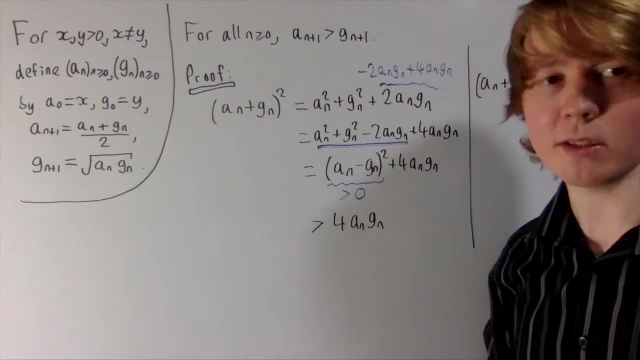 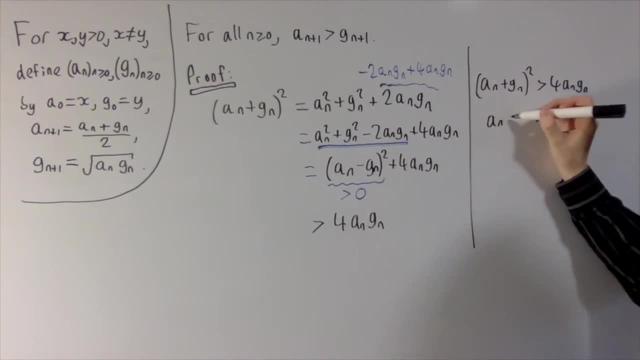 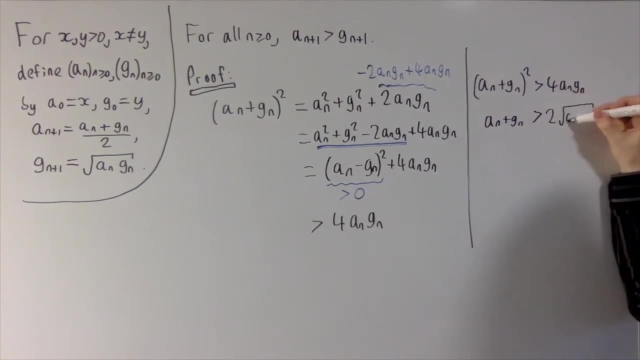 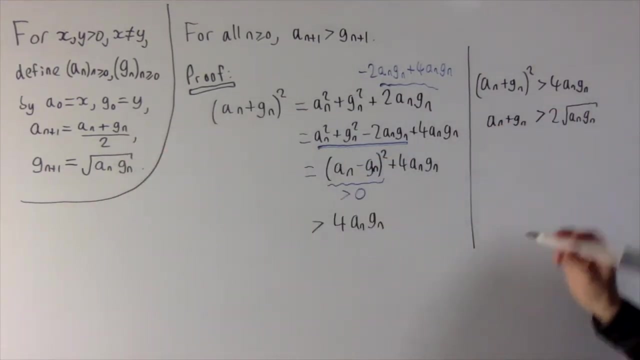 positive, so we can take the square roots of both sides here get: a n plus g n is strictly greater than the square root of all of this, which is 2 root a n, g n. And then we're almost in this sort of form with a n plus g n over 2, square root of a n, g n. We divide both. 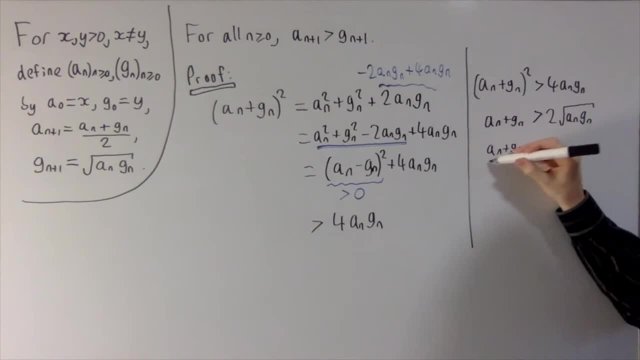 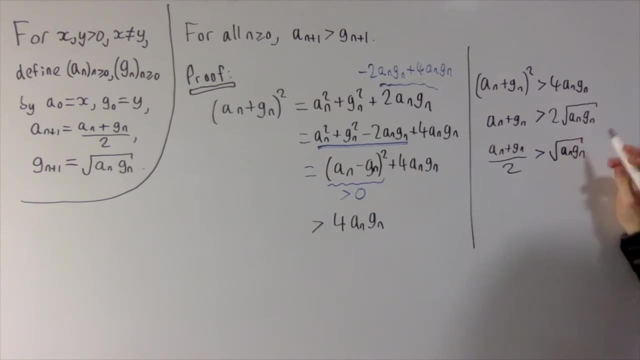 sides by 2, a n plus g n over 2.. This is strictly greater than the square root a n g n products there, And of course, this means that a? n plus 1 is strictly greater than g n plus 1, which is what we were trying. 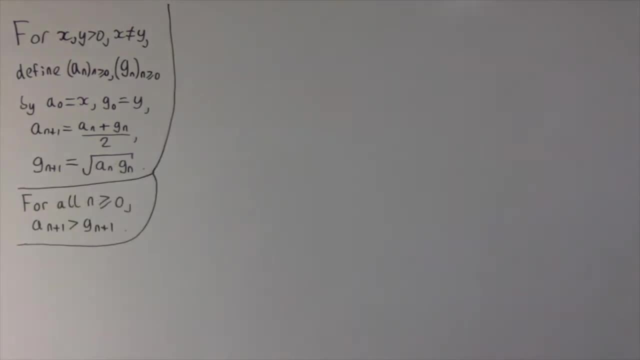 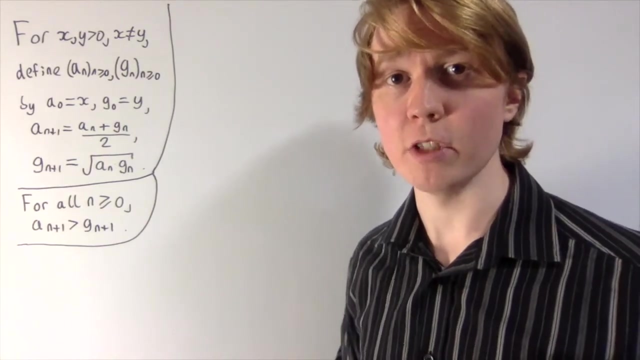 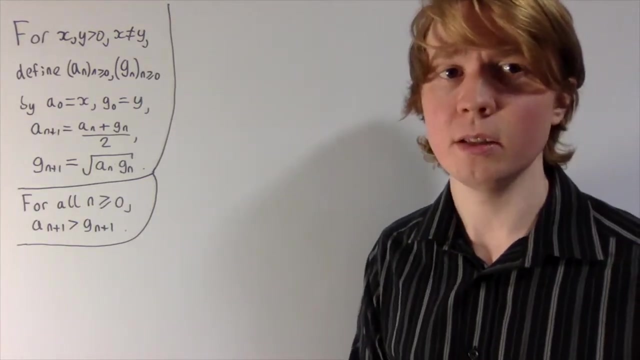 to prove there So this inequality, the fact that a n plus 1 is strictly greater than g n plus 1, this is actually a consequence of a more general result where, if you have any collection of numbers, so long as the geometric mean, the arithmetic mean, are both well-defined for these numbers, 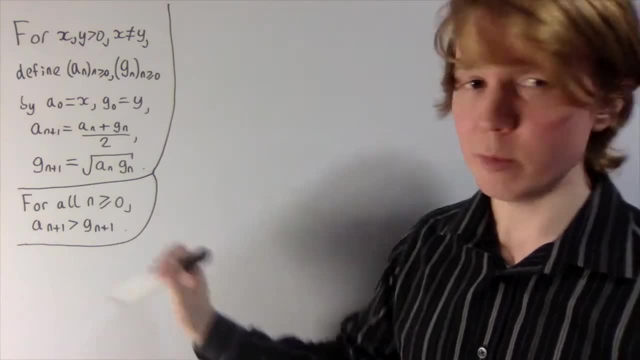 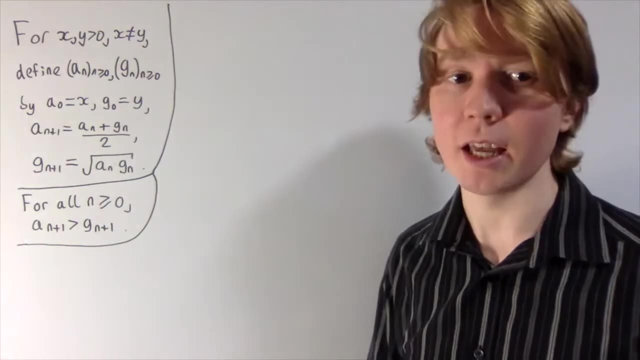 then as long as all those numbers aren't equal to each other, then the arithmetic mean will always be strictly greater than the geometric mean. So I guess we could have been a little bit more rigorous dealing with the strict inequality here, perhaps using proof by induction. 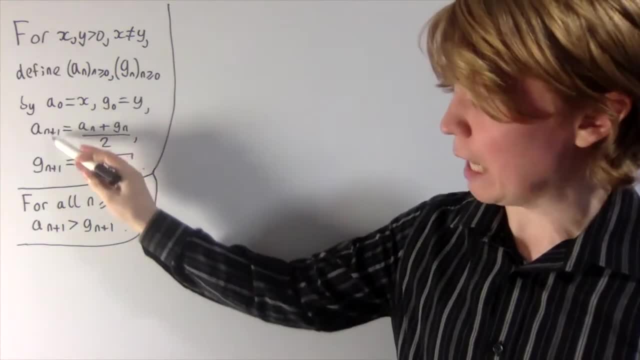 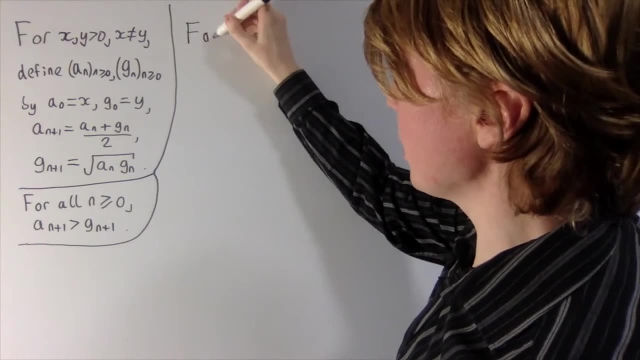 You can have a look at that if you're interested. So we're almost ready now to deal with limits, as n goes to infinity of these two sequences. But first we'll just have a look at the following property, which is that for all n plus g n, we're going to have a n plus g, n plus 1, square root of. 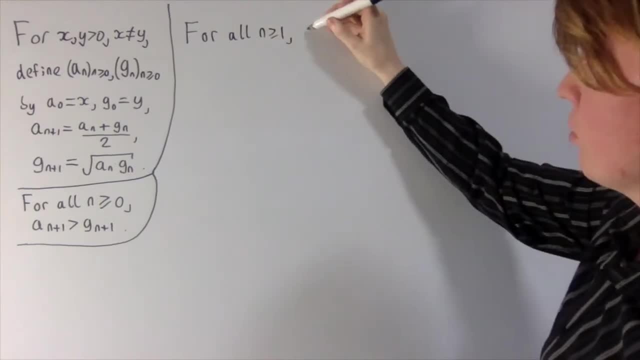 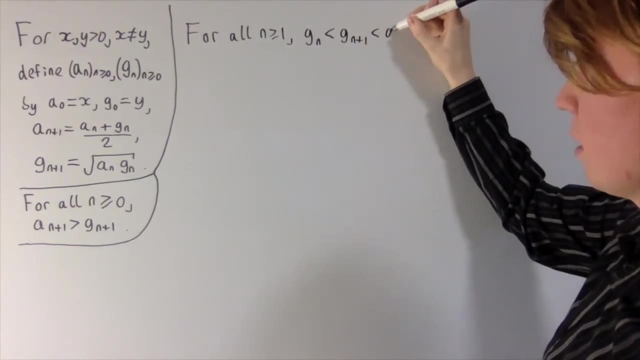 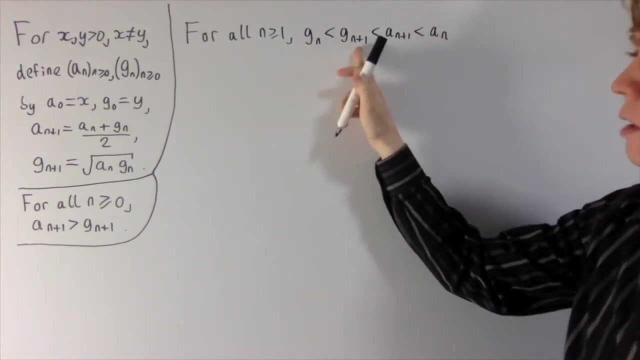 all n greater than or equal to 1, we're going to have a go at proving that g n is strictly less than g n plus 1,, which is strictly less than a n plus 1 is strictly less than a n. So what this means is our sequence- g is actually a strictly increasing sequence and our sequence 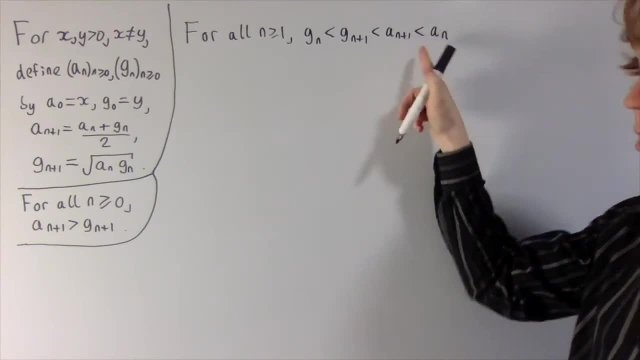 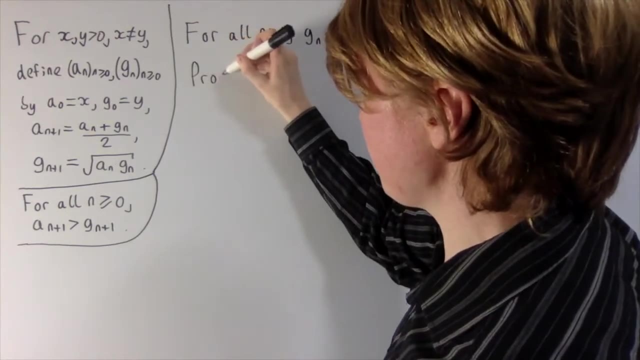 a. as you go from the nth term to the n minus 1th term, you're going down, and this is a strictly decreasing sequence. So this will turn out to be really useful. So we're going to go proving this. So, first of all, you'll notice- actually we've already done one of- 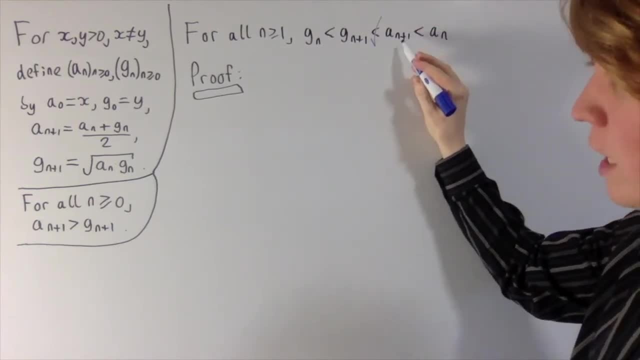 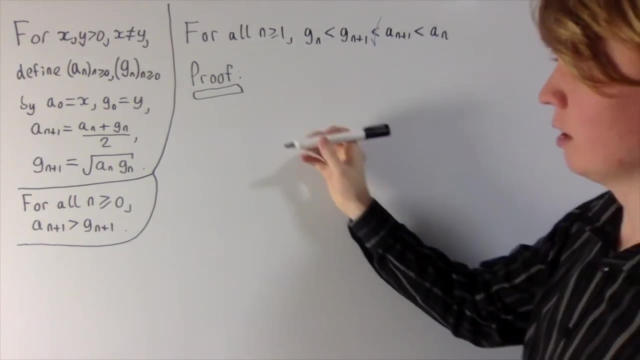 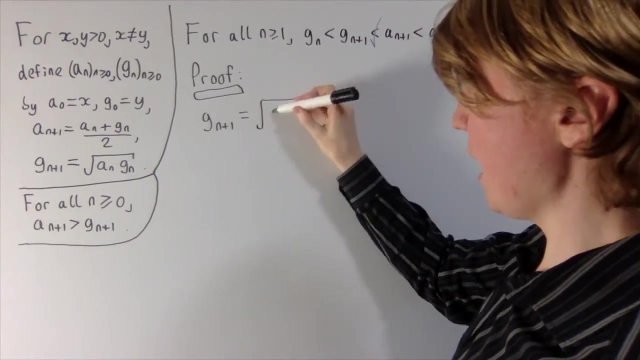 the inequalities. so I'll tick that off. We know that g n plus 1 is strictly less than a n plus 1.. So now let's try and show that g n plus 1 is strictly greater than g n. So let's write out what is g n plus 1.. Well, this is the square root of a n multiplied. 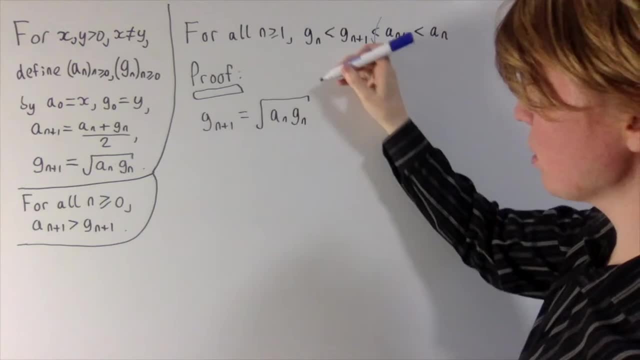 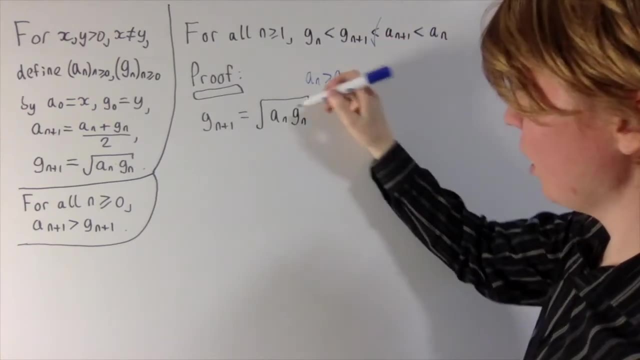 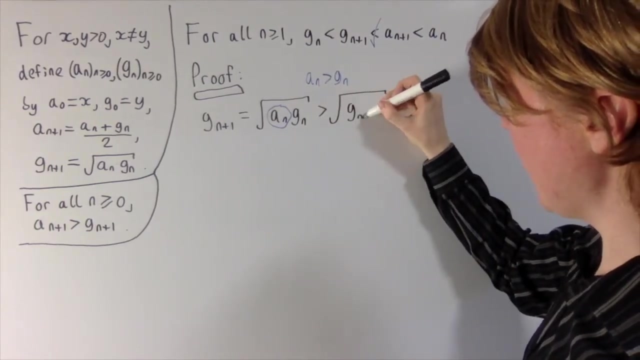 by g n. And here we know that. we actually know that a n is greater than g n, And what we can do then is replace this a n by a g n, And what we'll get is g n multiplied by g n. So here 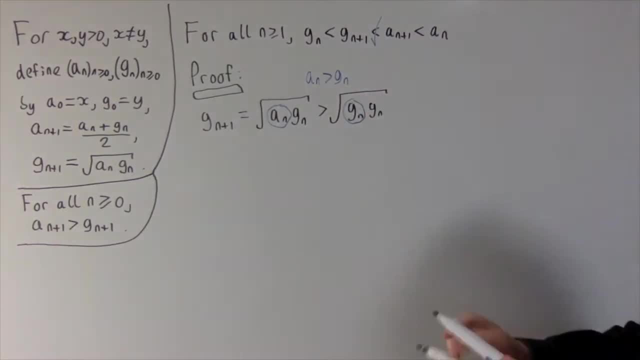 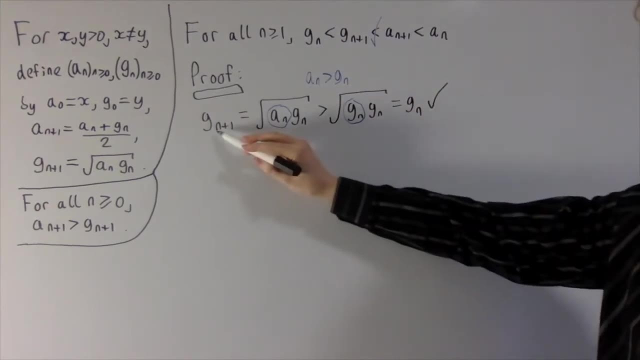 because we know that a n is greater than g n. replace this, we get a strict inequality. This here is just g n squared. The square root of that gives us g n. So g n plus 1 is indeed strictly greater than g n. So I'll tick this one off And then we can use a similar. 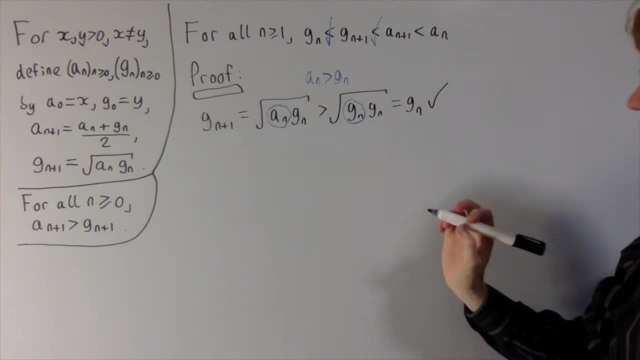 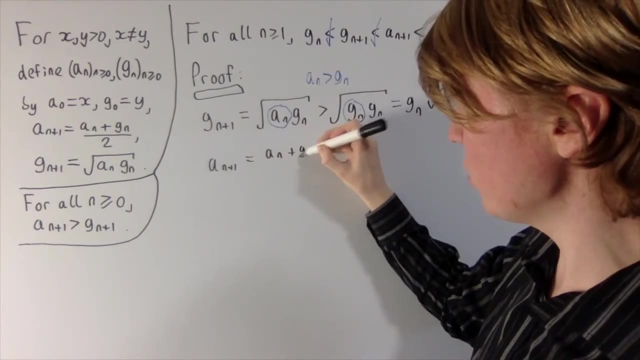 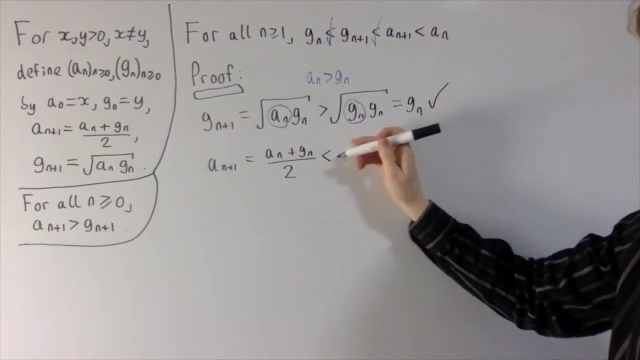 kind of approach for the inequality with a n and a n plus 1.. So what is a n plus 1?? This is the arithmetic mean of the previous two terms: a n plus g n. Divide this by 2.. And then, because we know that g n is less than a n, we can replace g n by an a n. here We'll. 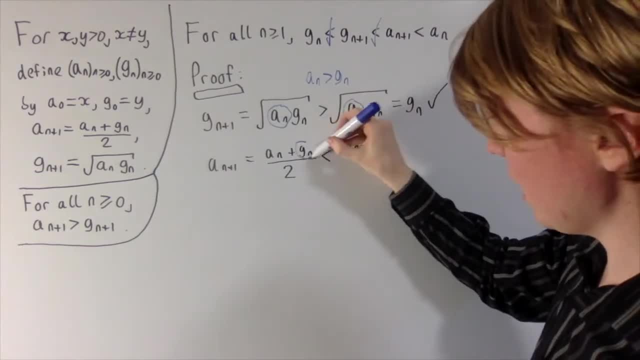 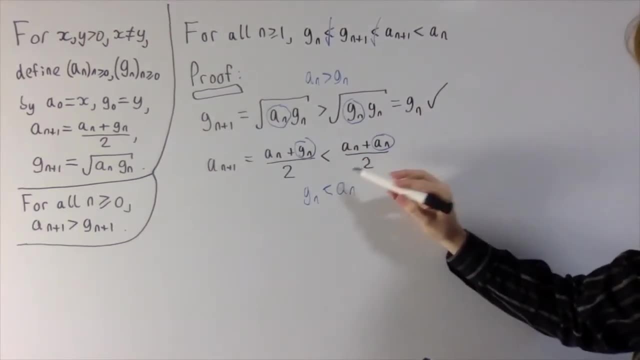 get a strict inequality. So here g n replace this by an a n. I know that g n is strictly less than a n. And then what do I get? a n plus 1 is strictly less than this thing, which is just 2 a n over. 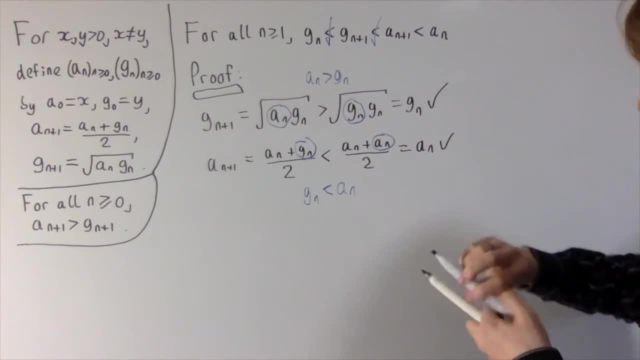 2,, which is a n. So that's what we were trying to prove there. So I can tick this off. And then we've shown all of these inequalities hold. So now let's put this inequality to use. So the first thing I'm going to do is draw. 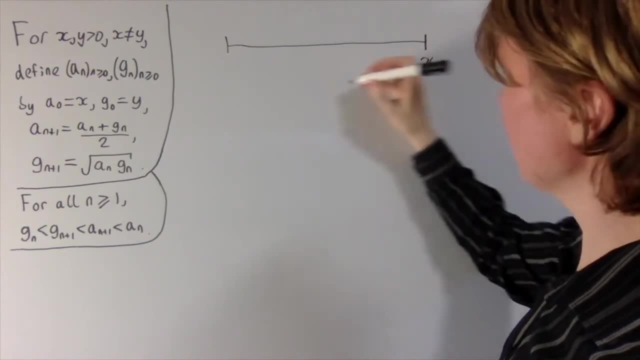 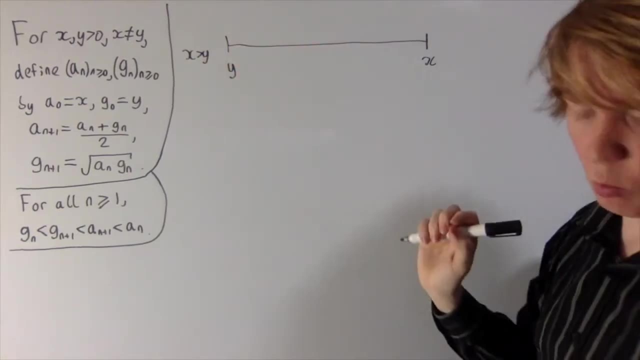 a graph about what's going on here. So let's assume that x is greater than y. So we'll deal with the other case in a sec. If we assume that x is greater than y, let's just have a look on the number line between y and x. what's happening with our a? n and our g? n? 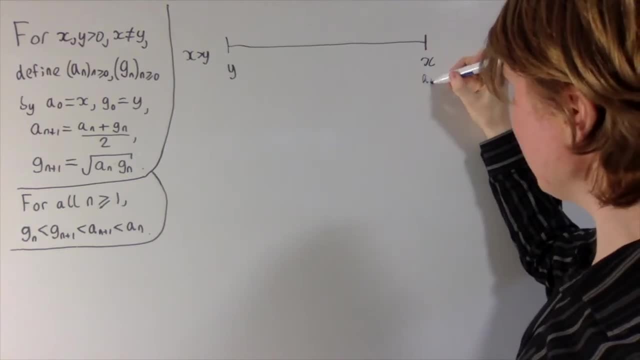 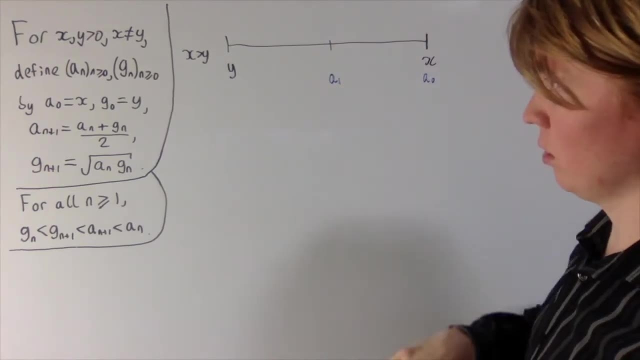 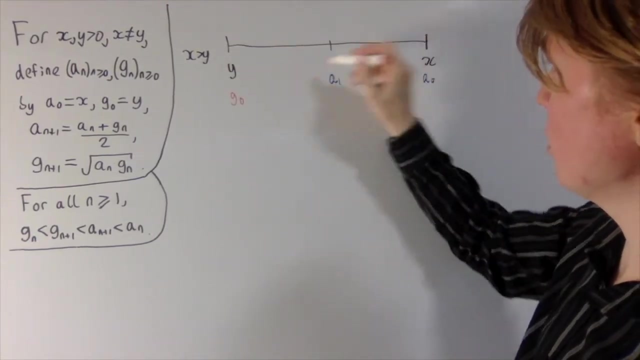 sequence. Well, we know that a 0 is equal to x, And we know that a 1 is the arithmetic mean of these two. We know that g 0 is equal to y, And then we know that g 1 is the geometric mean of y and x. This is somewhere between. 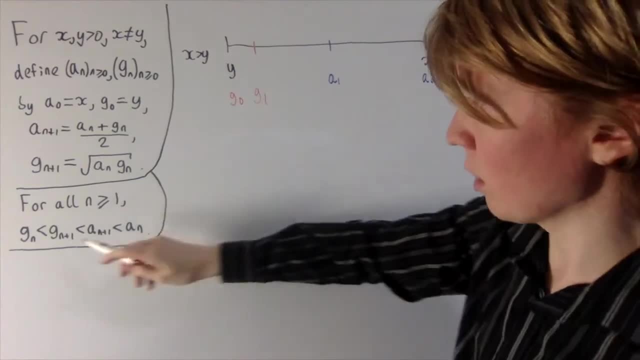 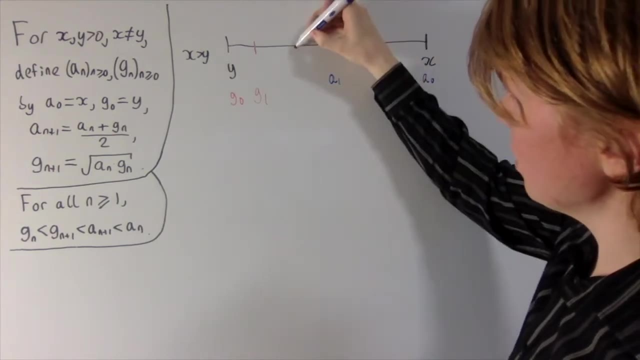 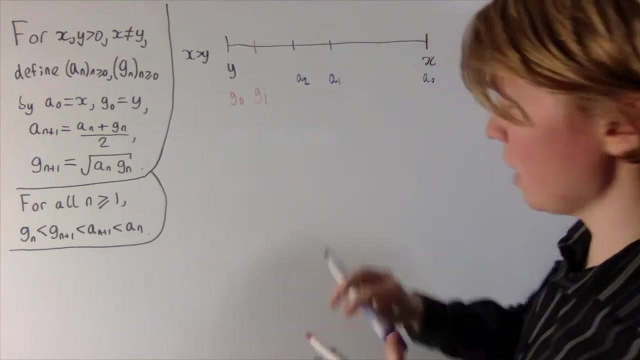 g 0 and a 1.. So we're using these inequalities here And then if we want to find the next term, if we want to find a 2, this is just the arithmetic mean, that's halfway between g 1 and a 1.. So a 2 goes here, And then to find g 2, this is going to be somewhere between 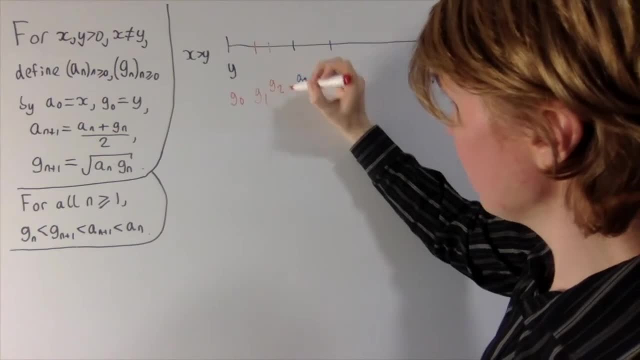 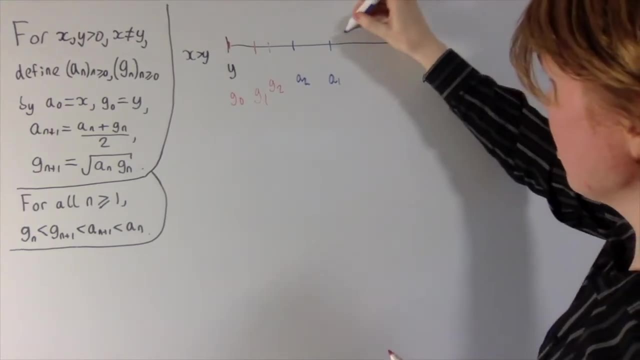 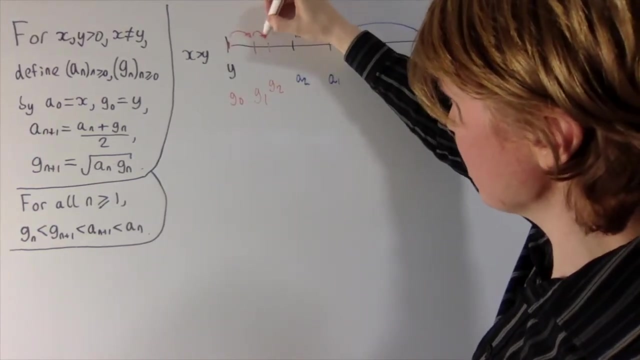 these, So maybe it's around here, So the kind of structure that we're seeing here. I also mark on g- 0 and a- 0.. So a is this decreasing sequence, g is this strictly increasing sequence? Perhaps, if I just put: 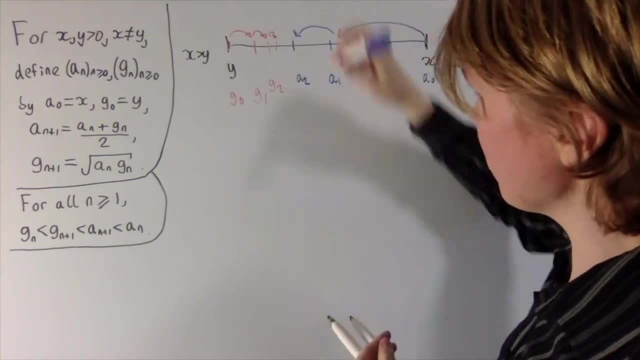 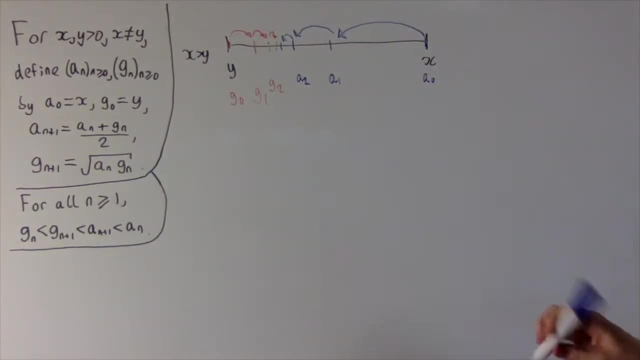 on another term. you can see. hopefully these two are going to coincide in the middle somewhere, And this should help us find the limits. OK, So I've assumed here that x is greater than y, So let's just have a quick look at what would happen if x was less than y. 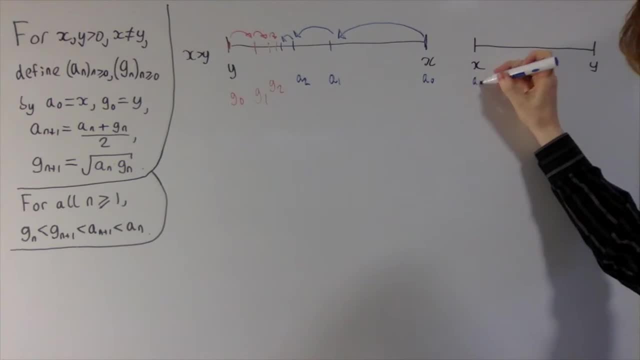 Then your a 0 would be all the way over here on the left, Your a 1 would still be the number in the middle between these two. Your g 0 would be over here on the right And your g 1 would still be somewhere around here. 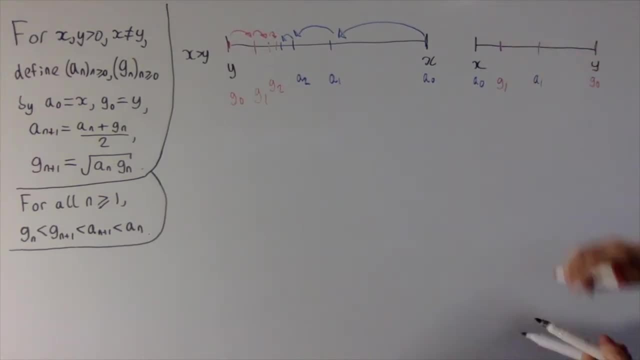 So what you'll actually find is from here to find g 2,, for example. this will be partway between g 1 and a 1.. Then to find a 2, this is going to be somewhere – it's halfway between g 1 and a 1.. So a. 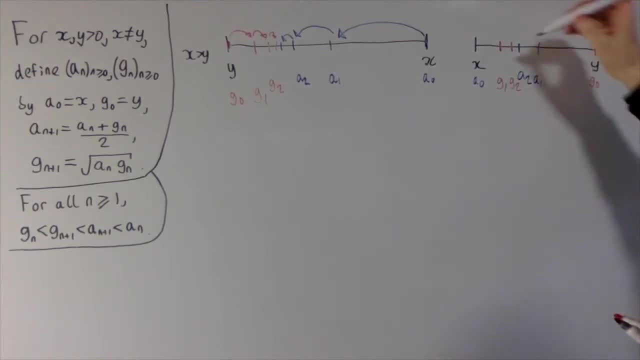 2 will be around here And then, if I just draw on what's happening with the arrows, So initially your a sequence would increase and then it would start decreasing very quickly, whereas here initially the G sequence would decrease, then it would start increasing. 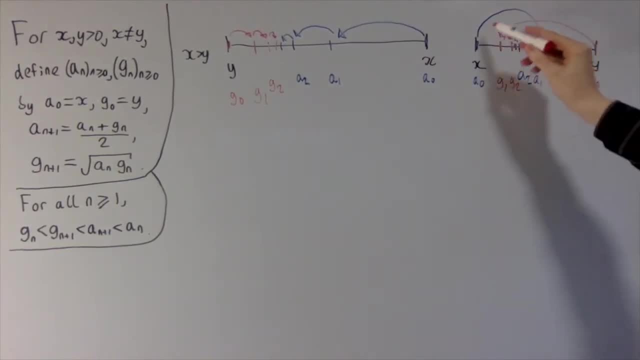 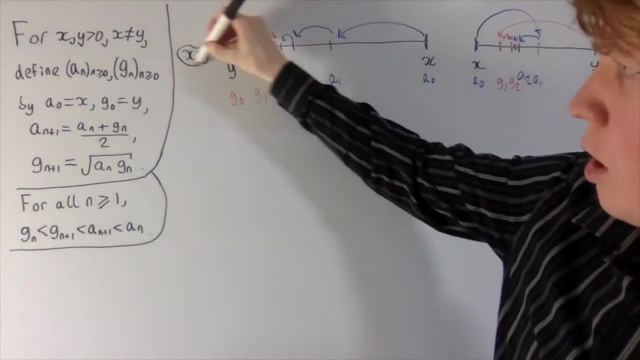 So you have this initial kind of crossing over, but actually, once this has happened after your first term, you've got this nice increasing, this nice decreasing property here. So let's deal with the limits now at long last. And how we're going to deal with this is using the monotone convergence theorem. 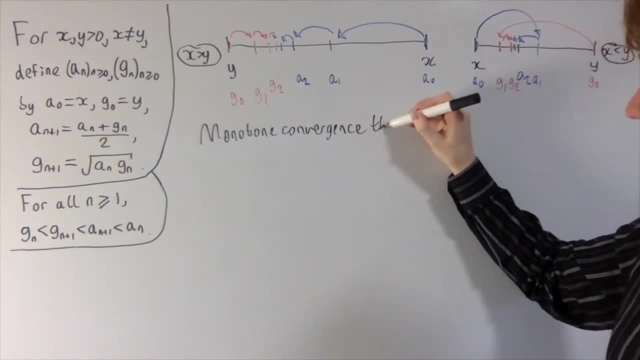 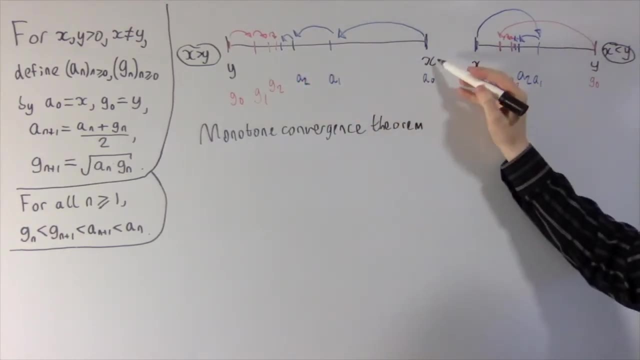 Because, if you notice, G is a strictly increasing sequence and it's bounded from above by either x or y, so bounded above by the maximum of x and y. And you'll also notice that A, our sequence here, is a strictly decreasing sequence, which is bounded below. 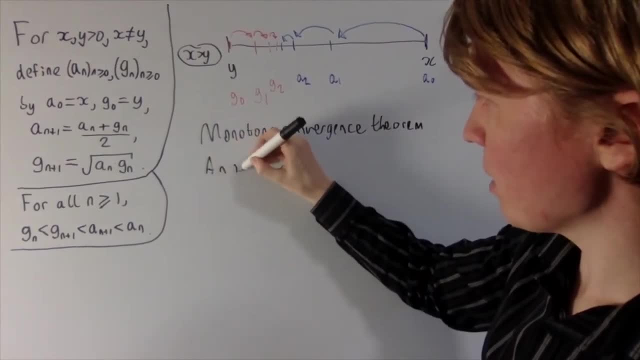 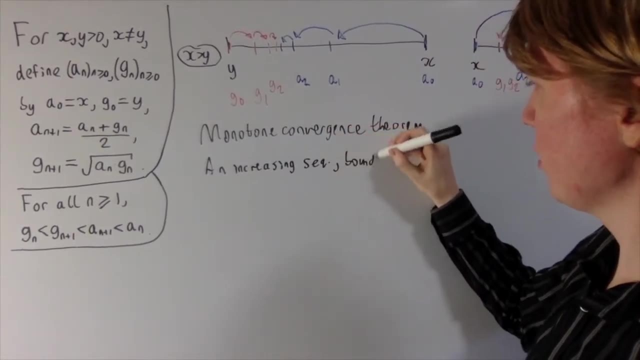 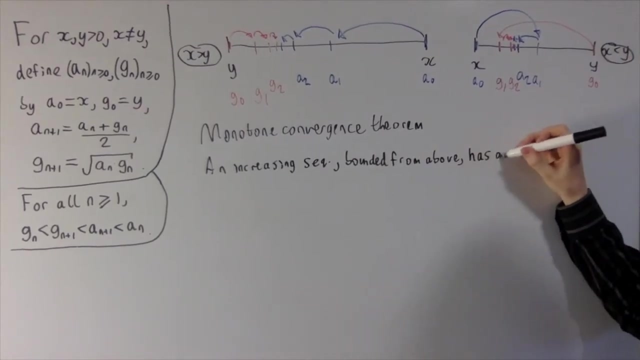 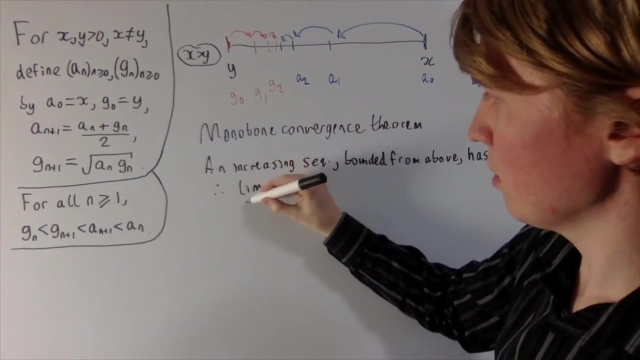 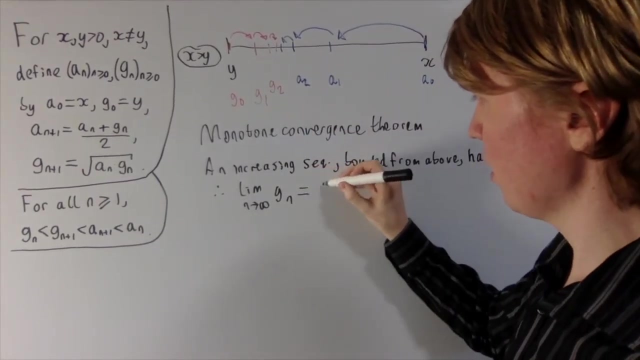 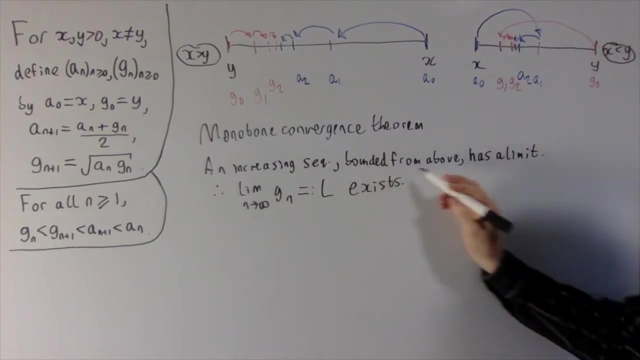 So if you have an increasing sequence which is bounded from above, this has a limit. So this tells us that the limit n goes to infinity of our increasing sequence. G exists And then we can call this L, And then similarly for a decreasing sequence bounded from below. 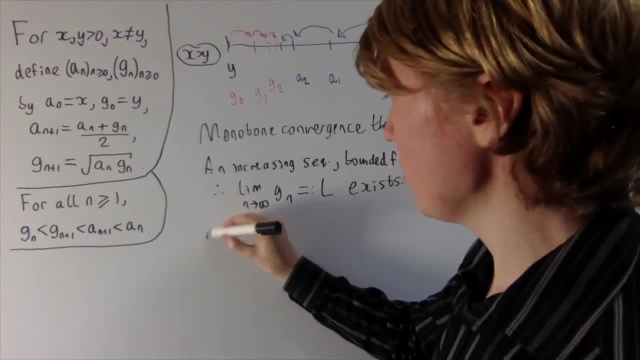 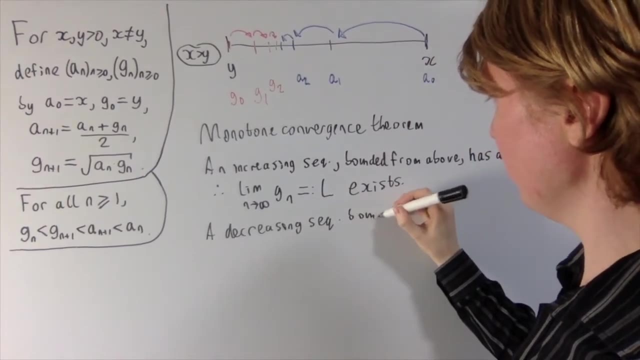 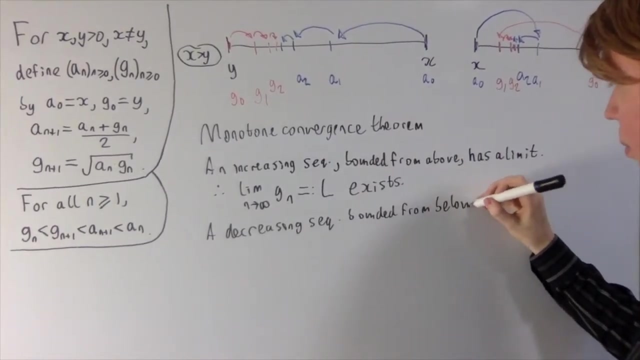 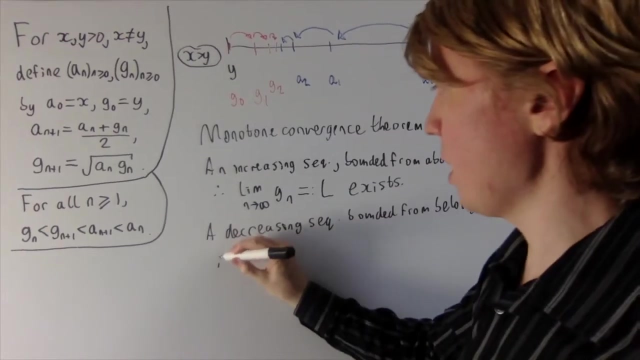 this also has a limit. So a decreasing sequence bounded from below. so here our A sequence is decreasing, it's bounded from below, by the minimum of x and y and this has a limit. So we can say that therefore. 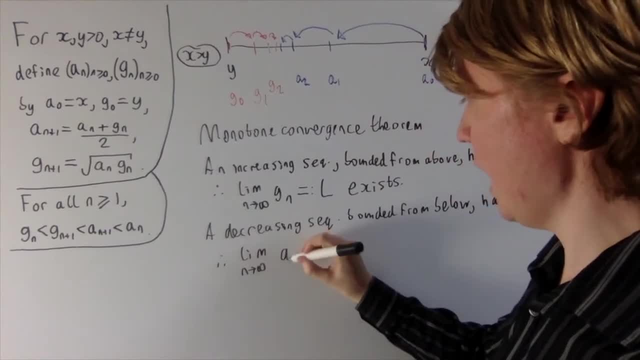 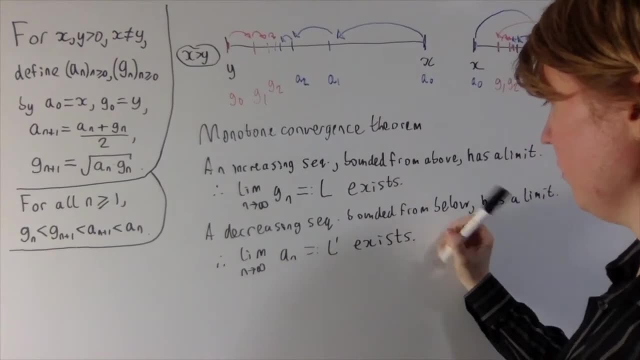 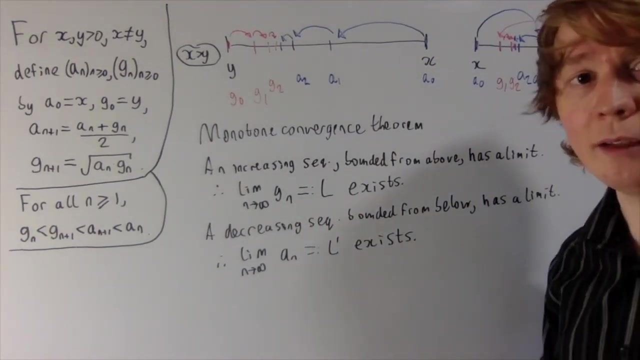 the limit, as n goes to infinity, A, we call this L' this also exists, But I can actually. I can go further than just saying that both of these limits exist, And this is where this example of the two sequences gets really interesting. 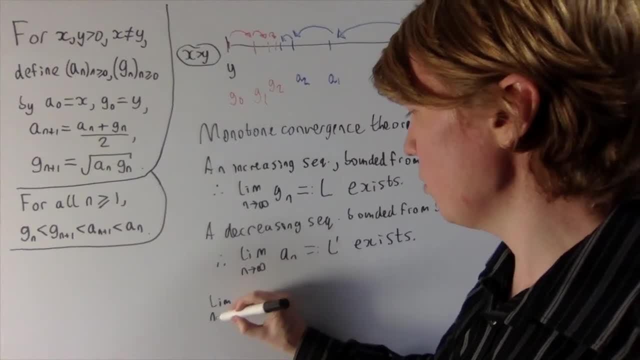 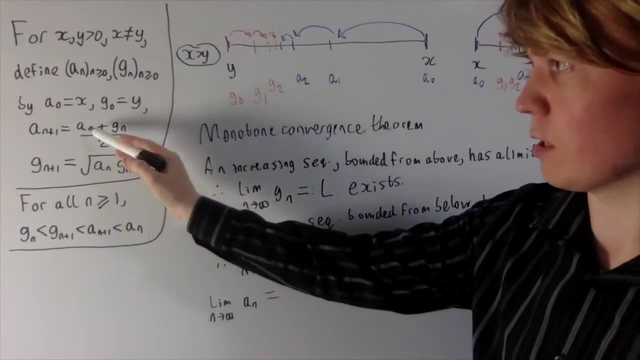 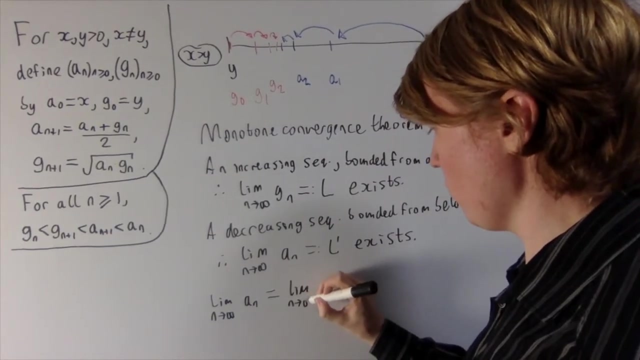 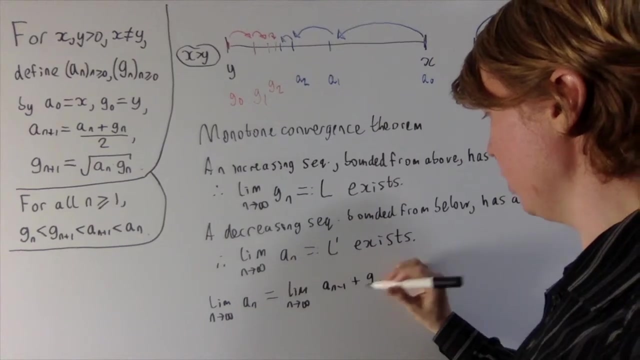 So the limit as n goes to infinity of A. well, I know that A this is going to be the same as A plus A plus G, So let's rewrite this as the limit as n goes to infinity: A plus G. 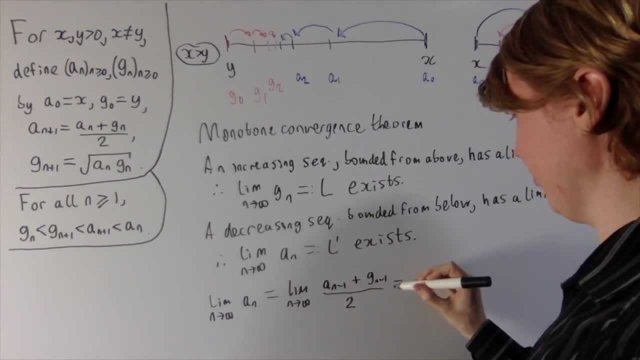 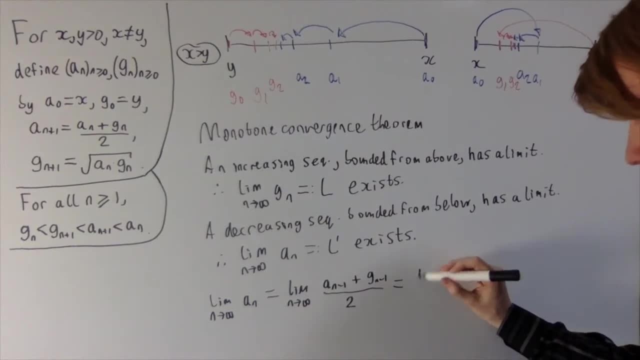 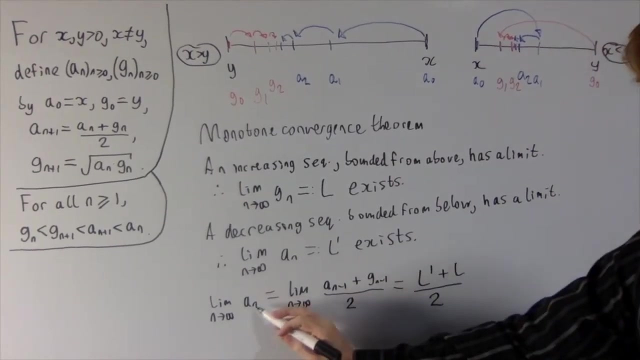 all over two. Well, we know that both of these sequences have limits, so we can use algebra of limits here. so this is actually equal to L dash plus L over two. But then we know that the limit as n goes to infinity of A. 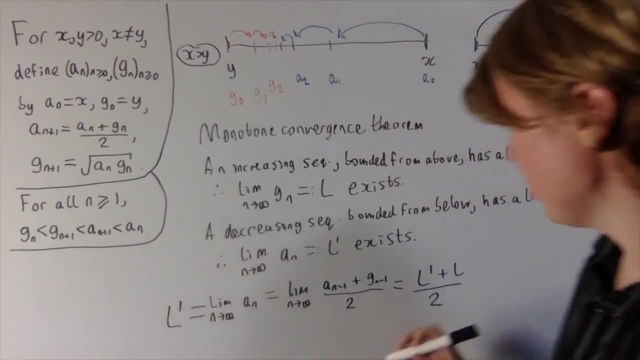 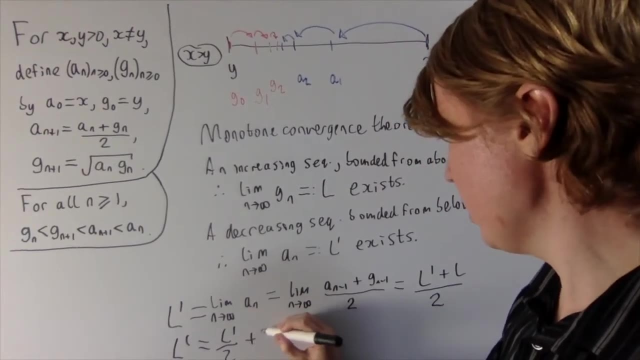 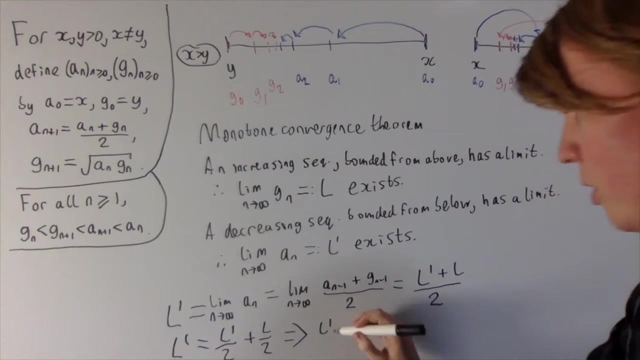 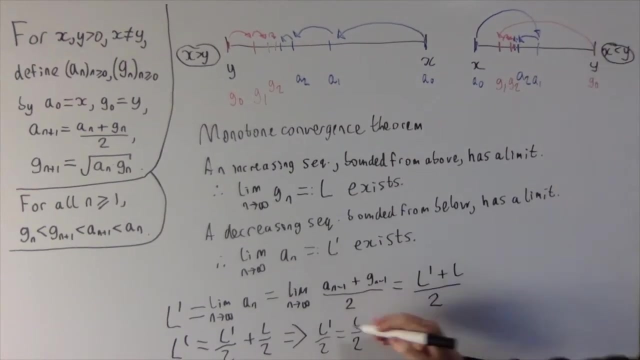 this is our L prime, so L prime is equal to L prime over two plus L over two. So this tells us that we subtract L prime over two from both sides, L prime over two equals L over two, and therefore L prime is equal to L. 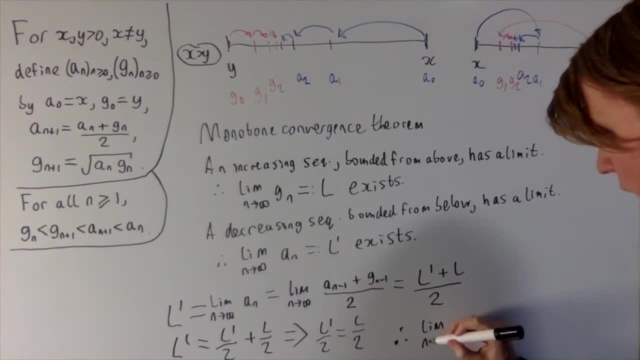 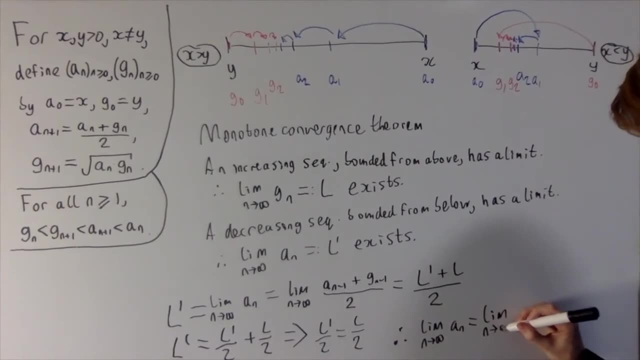 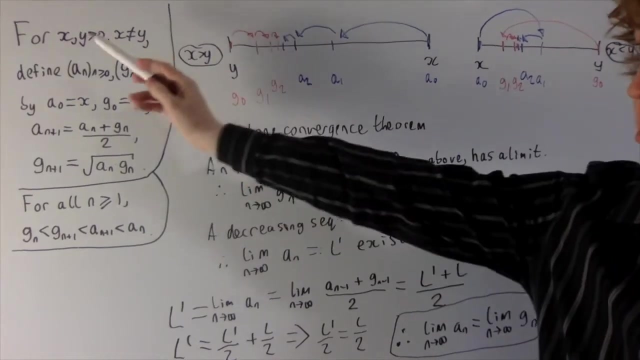 so we can conclude here that the limit as n goes to infinity of A is equal to the limit as n goes to infinity of our sequence G. So this is really nice. We've started with two distinct numbers, x and y. basically we keep finding the arithmetic mean. 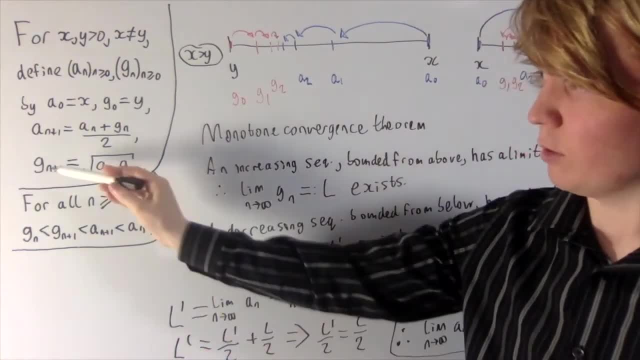 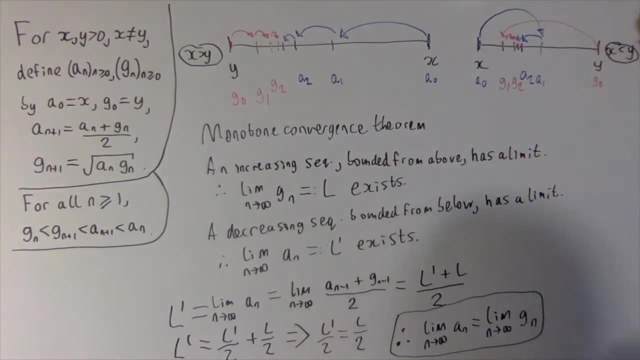 of the previous term in each sequence, and then for the G sequence we keep finding the geometric mean of the previous term in each sequence, and then eventually our limits will coincide here. So basically, we don't know exactly what this limit's going to be. 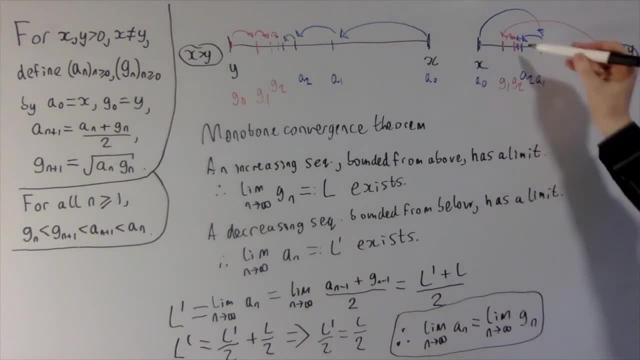 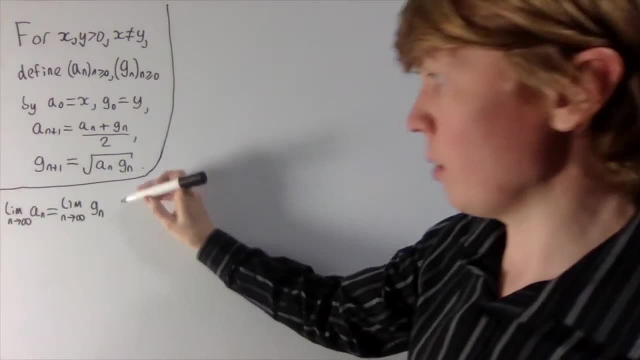 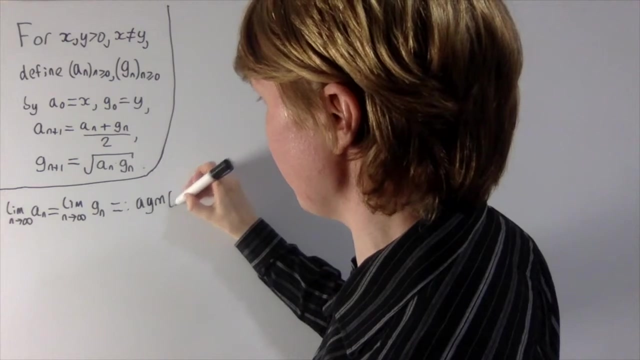 there's no particularly nice way of calculating it, but we know that this limit exists and these two do coincide. So the payoff of showing that these limits exist and are equal is that this common limit gives rise to something called the arithmetic geometric mean of two numbers, x and y. 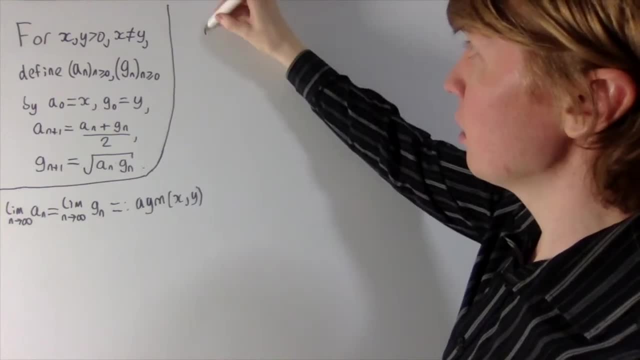 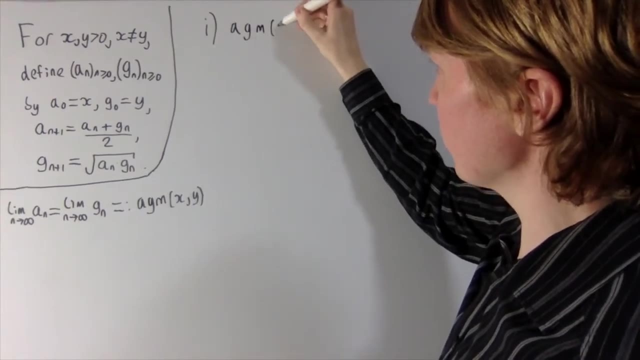 You can also call this the AGM of x and y. So as a payoff of showing that this thing exists, we'll have a look at a couple of properties quickly. So the arithmetic geometric mean is symmetric. What that means is the AGM of x- y. 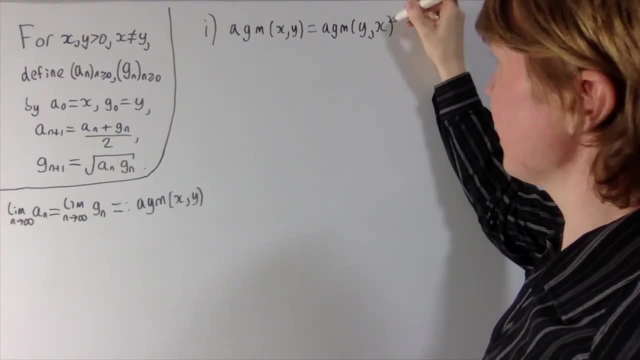 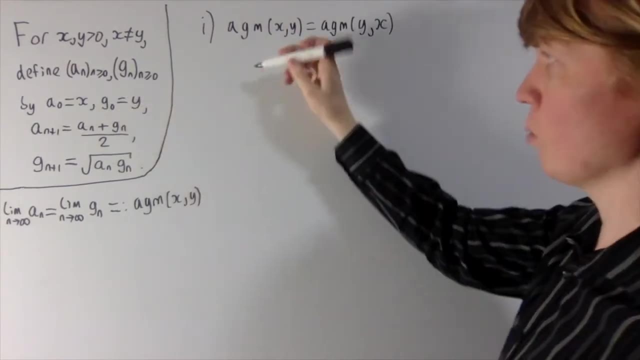 is the same as the AGM of y and x. And you can see this because if you imagine you've got different a0 and g0, you just swap your x and y around, but here a1, this would be equal to. 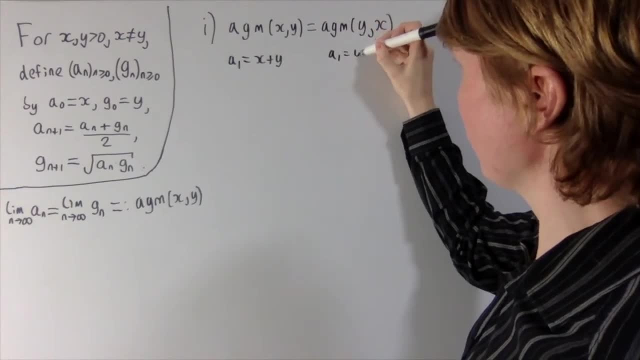 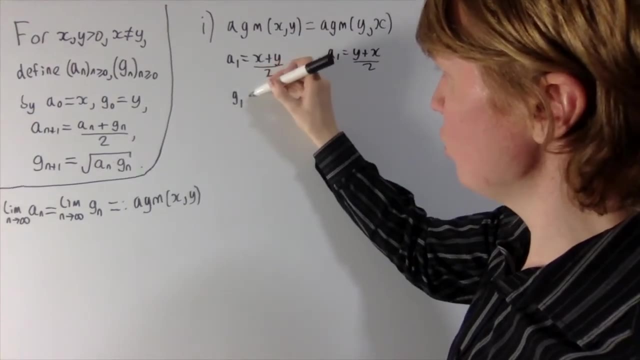 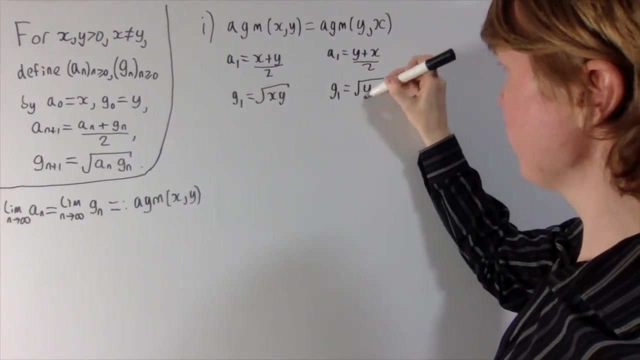 x plus y. Here a1 would be equal to y plus x, and both of these divided by 2.. And here g1, this would be equal to root x- y, Whereas here g1 would be equal to root y- x. 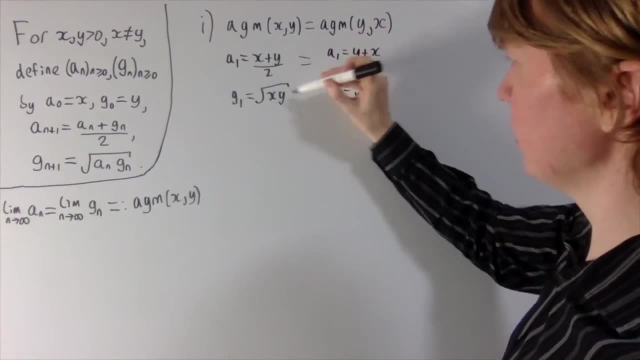 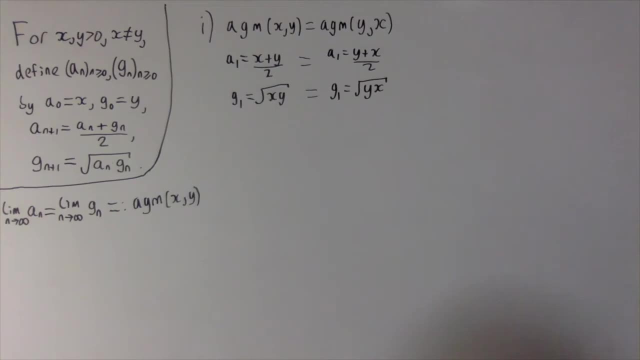 Of course, x plus y, y plus x, these are equal. Here, root x, y, root y x, these are also equal. So this is symmetric. it doesn't matter which way around you have your x and y. 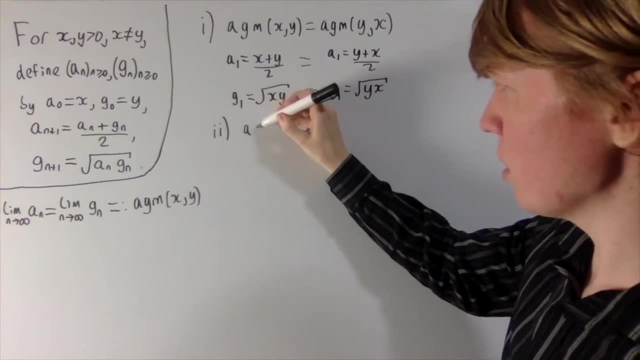 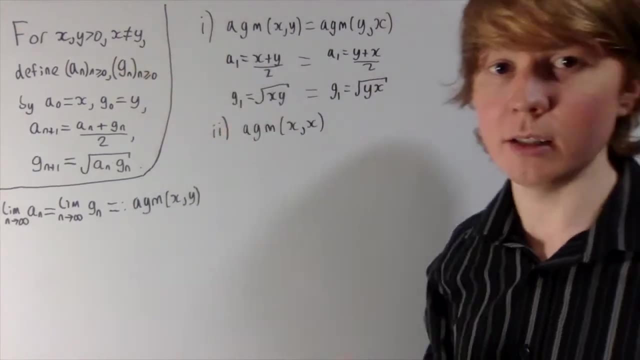 So another property we'll have a look at here then is if we kind of try and extend the definition a bit. So initially we assume that x and y aren't equal. What would happen if you had the quadratic geometric mean of x and itself? 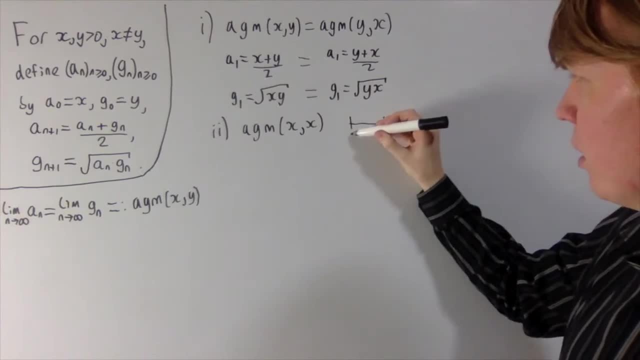 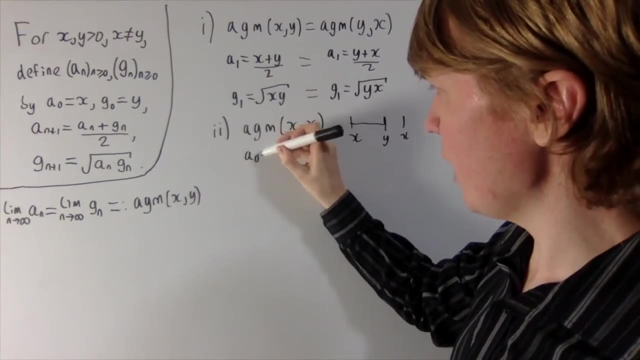 Well, kind of pictorially, your number line, instead of being between x and y, you just sort of start at the point x, And here you'd have a0 equals g0 equals x, a1, this would be equal to. 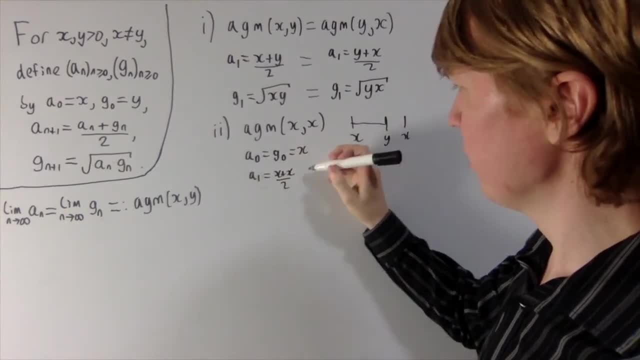 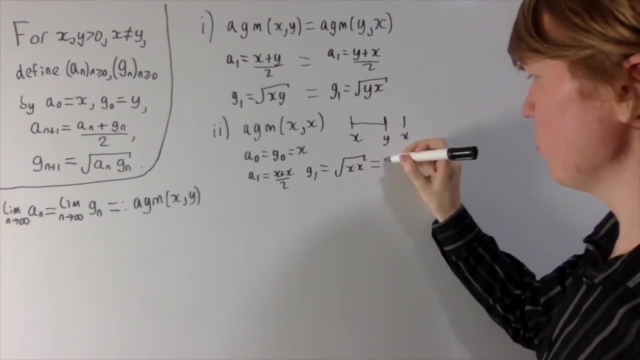 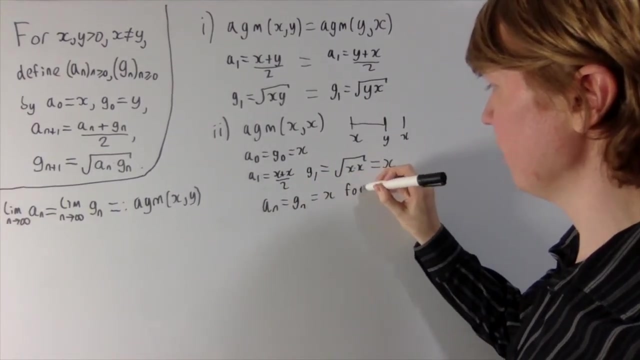 x plus x over 2. g1, this would just be equal to root x times x. so root x squared This would be equal to x. So actually a1 would be equal to g1 would be equal to x for all n. 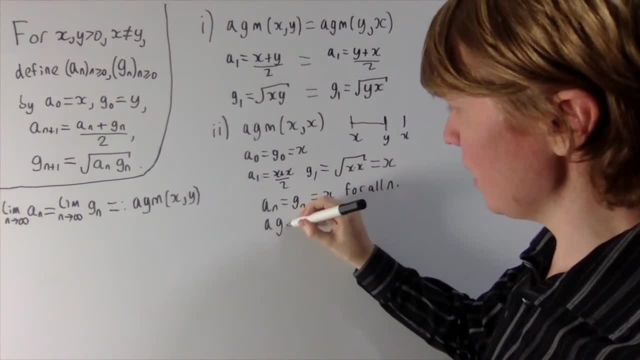 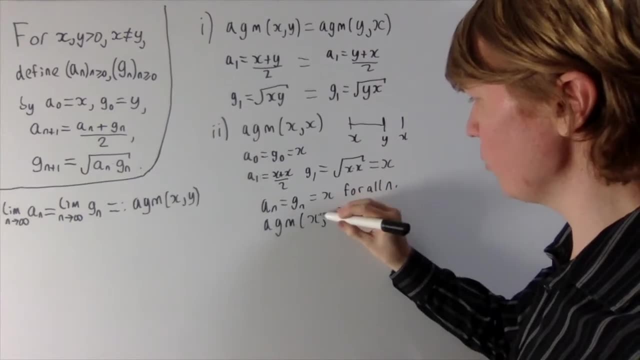 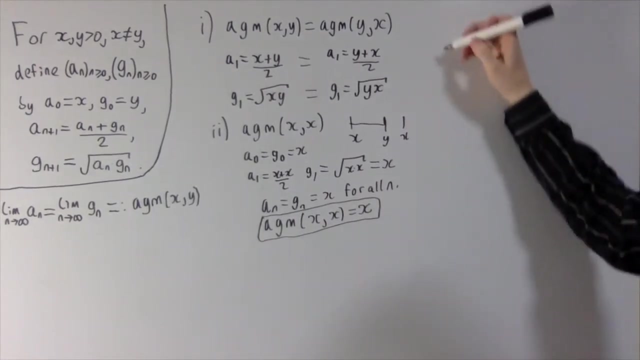 So what this means is the a1 of x and itself would be equal to x, which is a nice property to have. if you have any sort of mean of a number and itself, you should get that number back. So another property we'll have a look at. 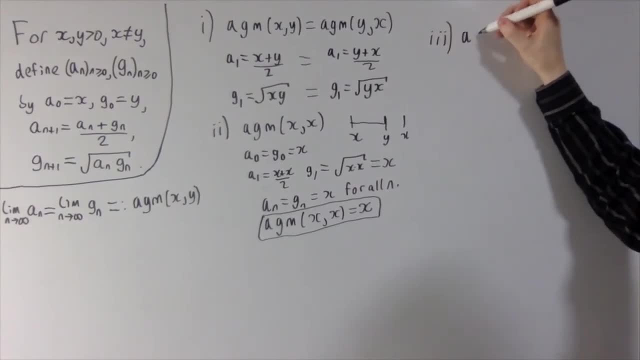 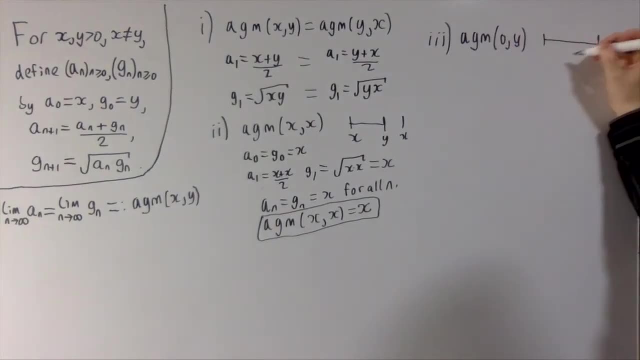 So again, try and extend the definition a little bit here. What would happen if you had the arithmetic geometric mean of 0 and y? So in our picture here, imagine you have 0 and y, Your starting point, well, g of 0,. 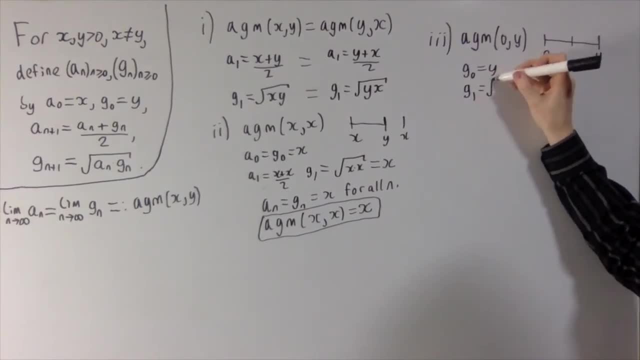 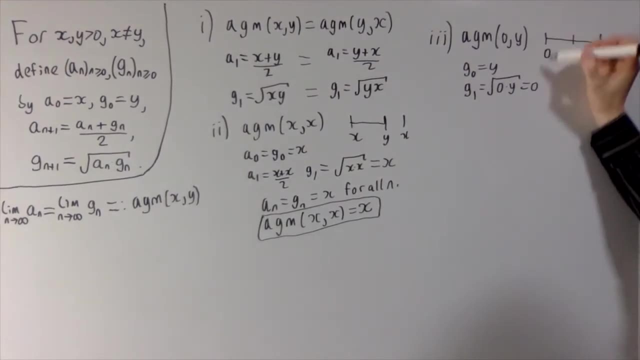 this would be y, Then g of 1, this would be the square root of 0 times y, which would be 0. So g would basically just be equal to 0. And then, however many terms you go in, you'll find that. 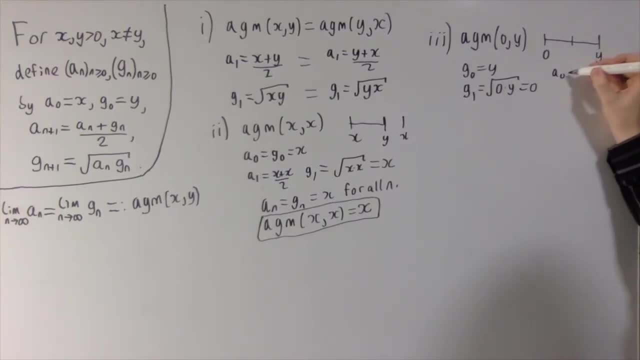 gn is always going to be equal to 0. So a0,, this would be equal to 0.. a1,, this would be equal to y over 2. You do 0 plus y over 2. a2, then this would be y over 4,. 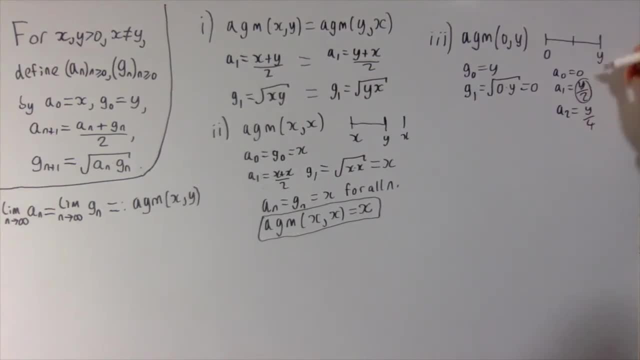 because you would do the arithmetic mean of y over 2 and 0. So kind of what happens with your a is you've got this decreasing sequence which will just decrease down to 0. So here you can say your agm of 0 and y is always equal to 0. 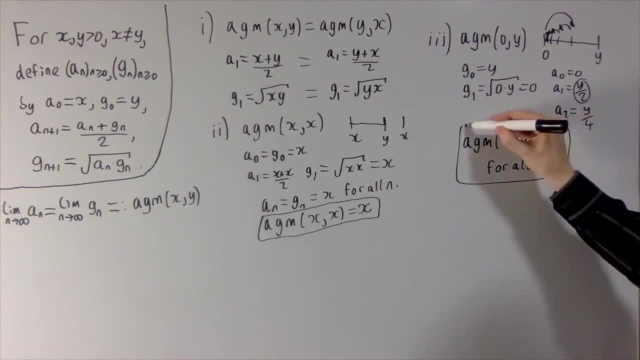 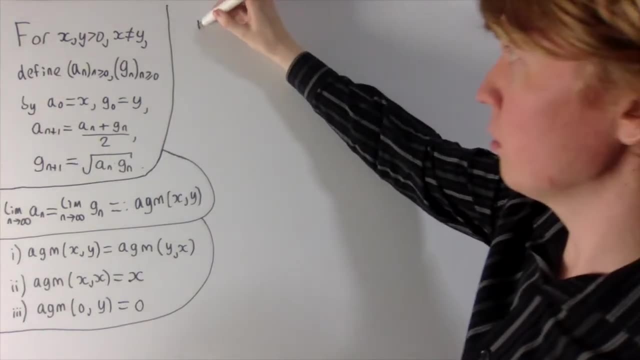 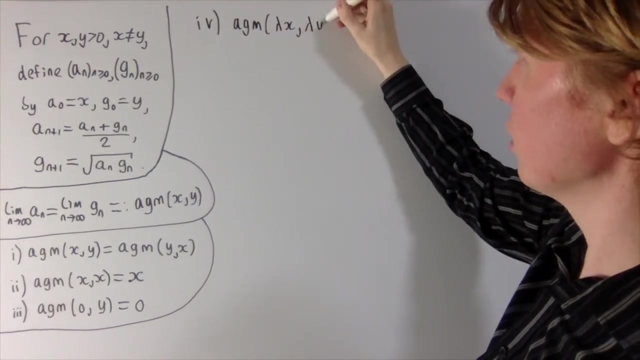 for all y. So finally, let's have a look at one last property of the arithmetic geometric mean, which is that it preserves scalar multiplication. So if you have the agm of lambda x and lambda y, this is always the same as lambda multiplied by. 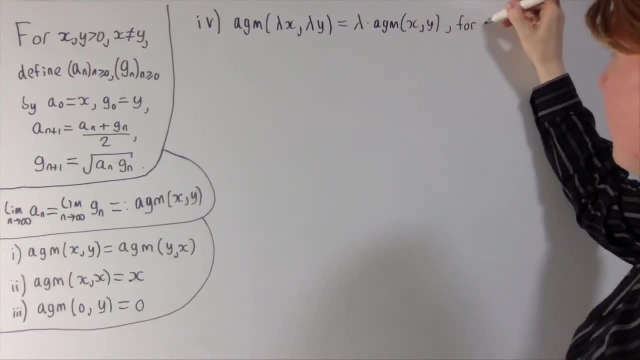 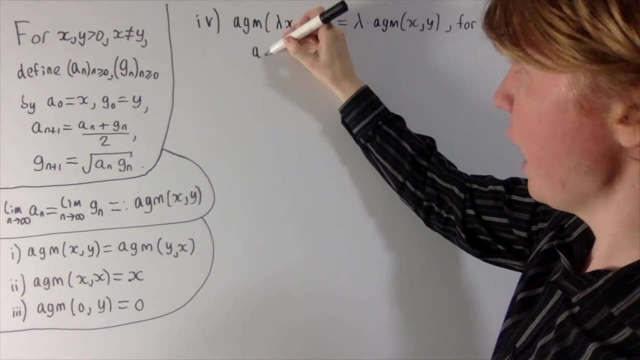 the agm of x and y for all lambda greater than 0.. And in fact you can go even further to say that if you have an lambda you call it, and if you call this gn lambda, so your two sequences where you've got the lambda inside. 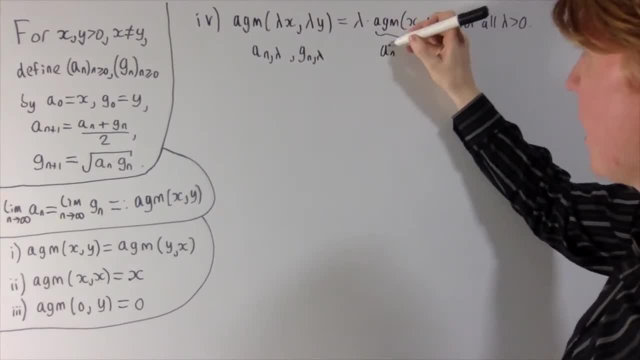 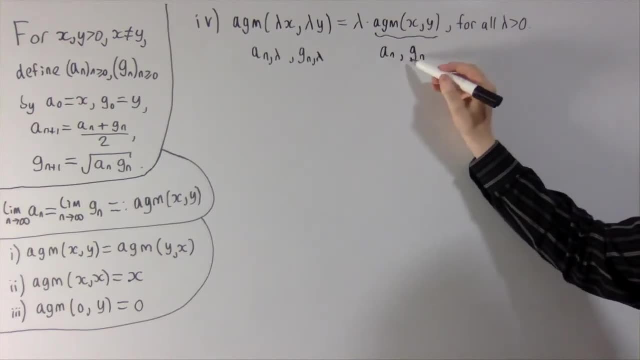 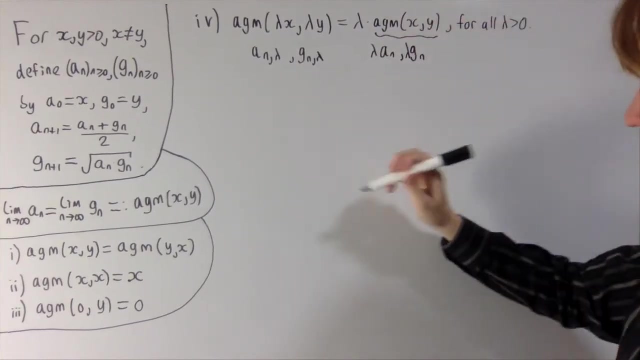 versus for this sequence. if you just call this an and gn, as before, then in fact an lambda is always going to be equal to lambda an and gn. lambda is always going to be equal to lambda gn, And we can prove this by induction. 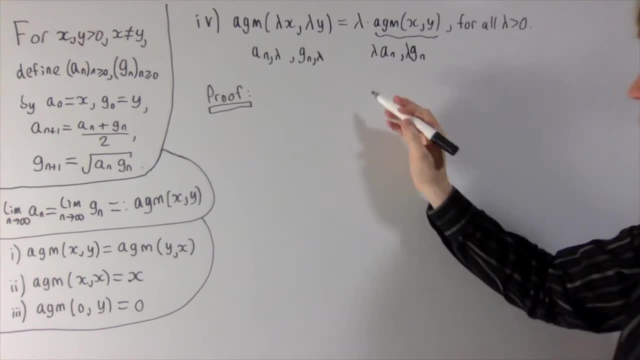 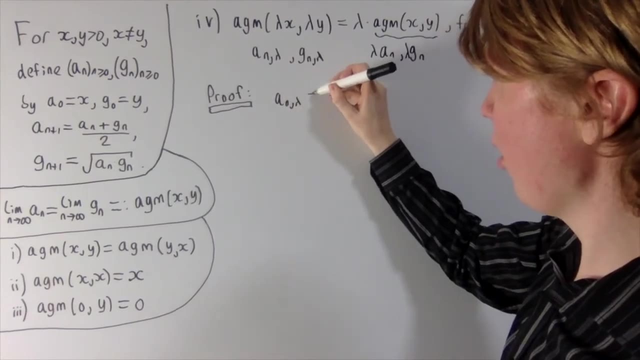 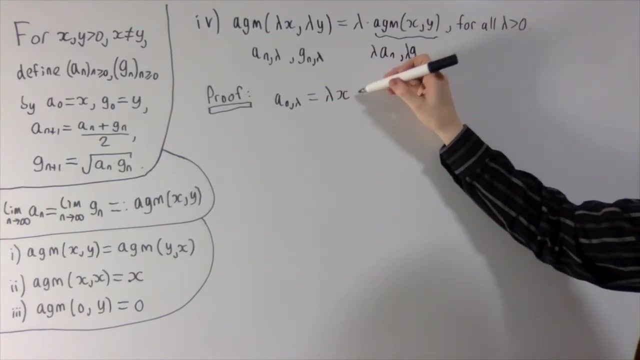 So let's just start off with a0, lambda, g0 lambda show that these are equal to lambda a0, lambda g0.. So a0- lambda- this is the first term in this sequence, which is just lambda x And then lambda x. 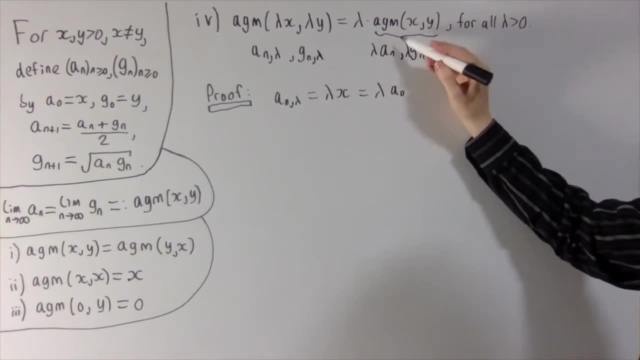 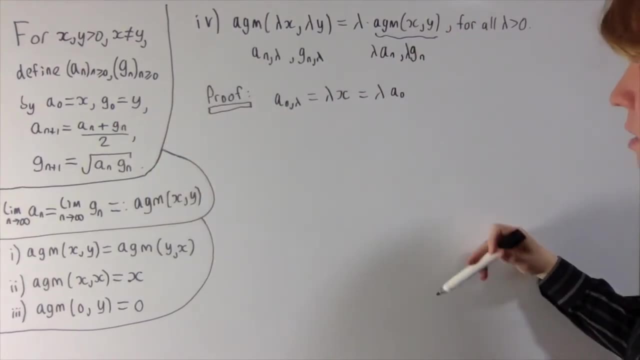 well, this is just lambda times a0, where the first term in this sequence, because we've got x there, our a0 is just equal to x. So a0 lambda is equal to lambda multiplied by a0.. And then similarly. 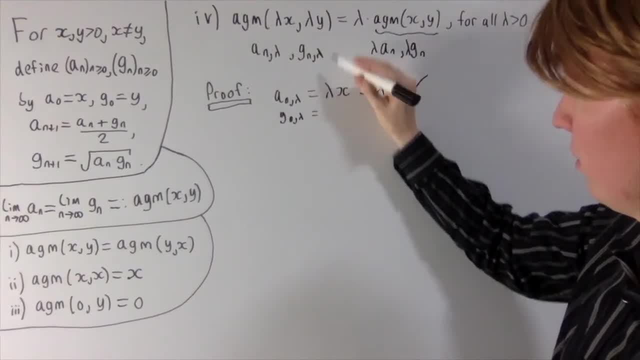 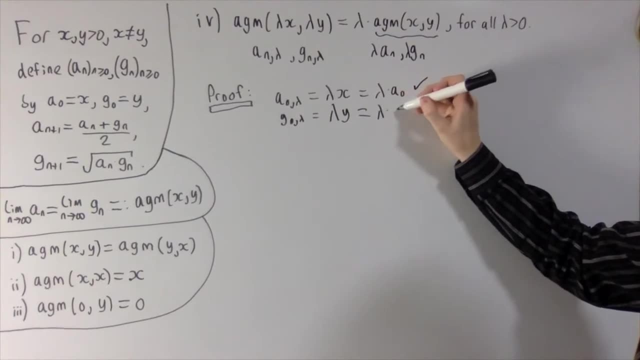 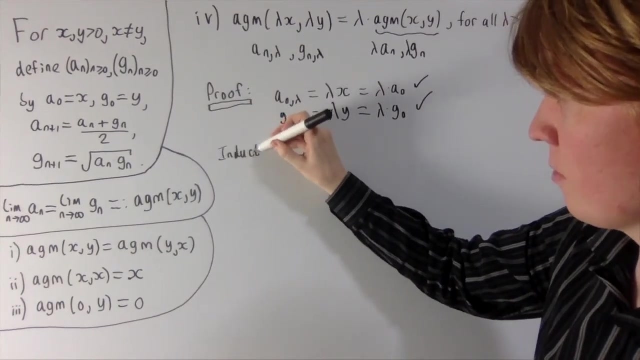 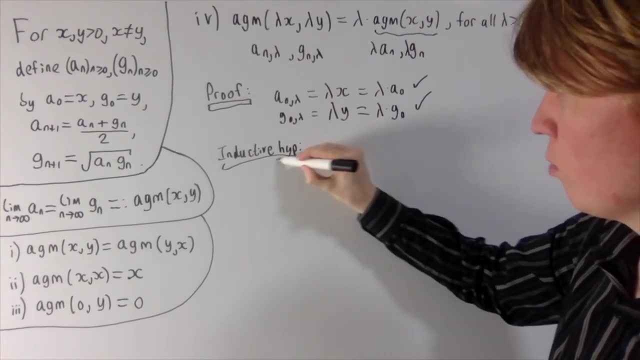 g0- lambda- this is your first term here- is lambda y, Then your first term here is just y in the g sequence. So this is lambda times g0.. So our inductive hypothesis then we'll just assume that these are equal for n minus one. 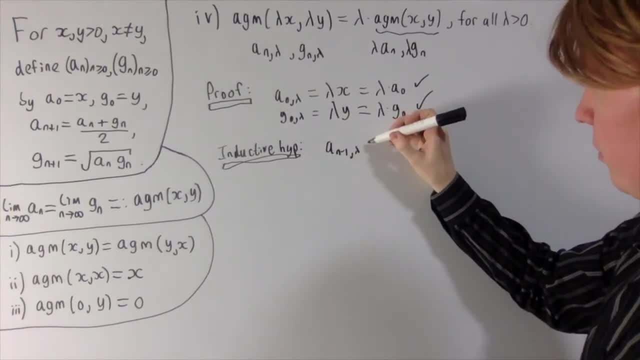 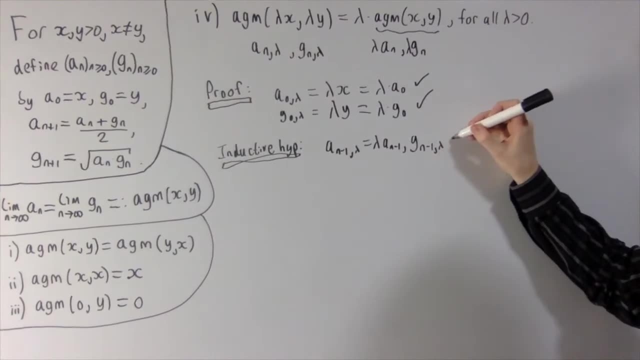 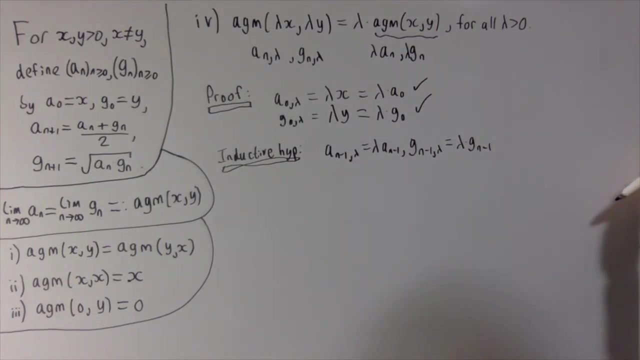 We'll say that an minus one lambda is equal to lambda an minus one, And also gm minus one lambda is equal to lambda multiplied by gm minus one. So now, what we'll do is we'll try and prove that these are equal for all. n. 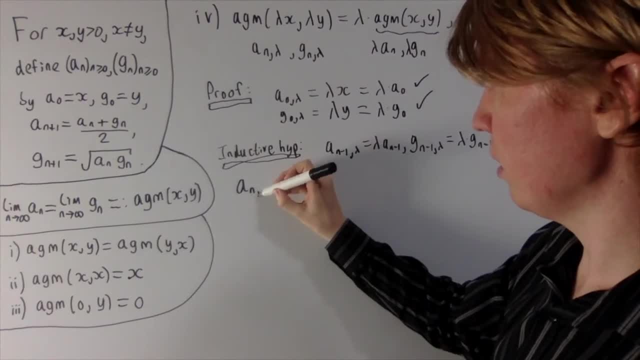 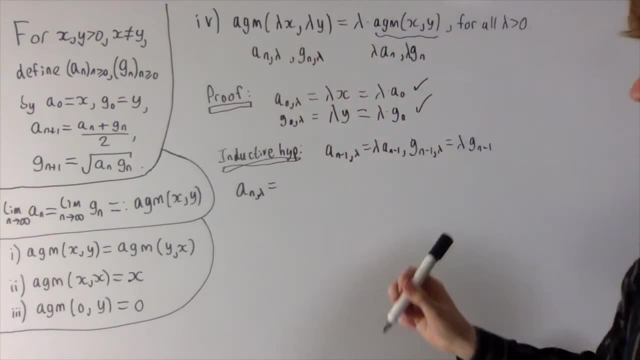 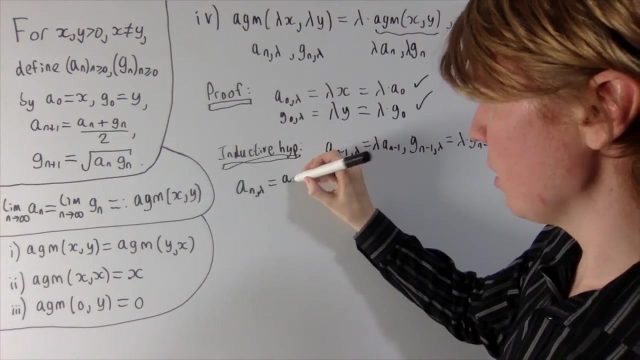 using the inductive hypothesis. So now an lambda. So this is the nth term in the a sequence where we started with lambda. So what is this? Well, we just add together the previous two terms from each sequence and divide by two. So this is an minus one lambda. 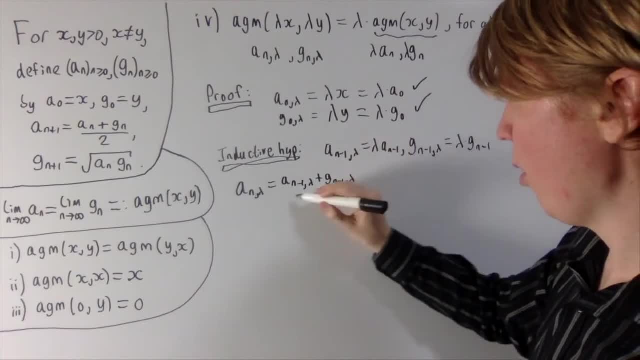 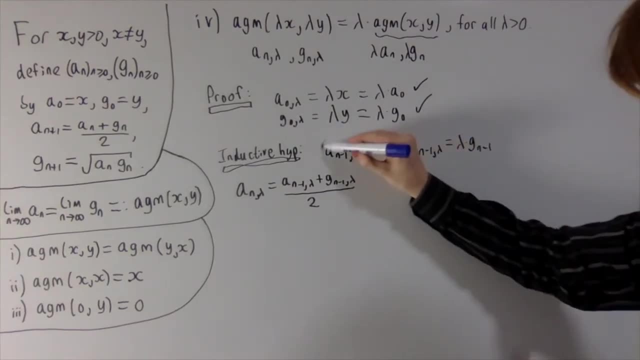 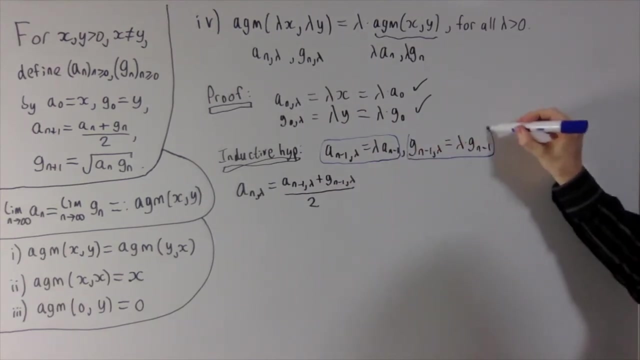 plus gn, minus one lambda, all divided by two. But then, using the inductive hypothesis, we know that an minus one lambda is equal to lambda times an minus one for the other sequence And similarly for g. So actually we can replace both of these straight away. 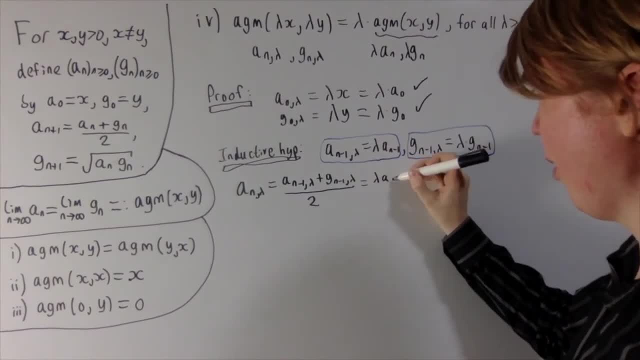 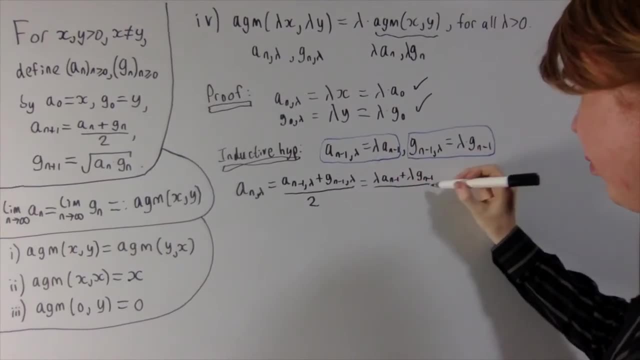 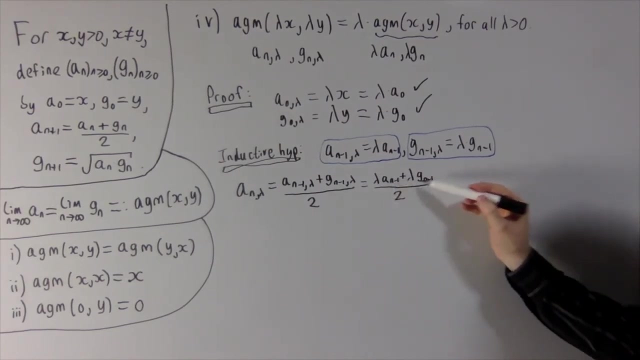 by this is equal to lambda an minus one plus lambda, gm minus one, all over two. Then taking out a factor of lambda here you'll see you've got lambda multiplied by an plus one plus gm minus one plus gm minus one, all over two. 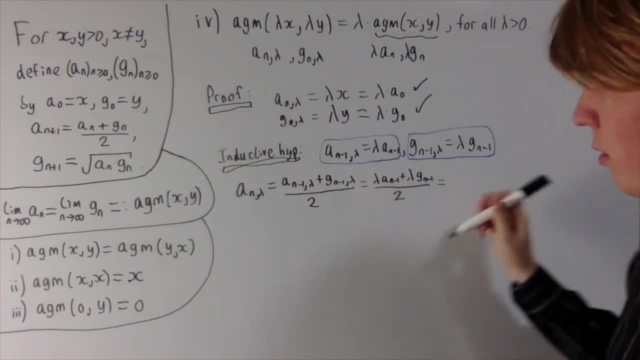 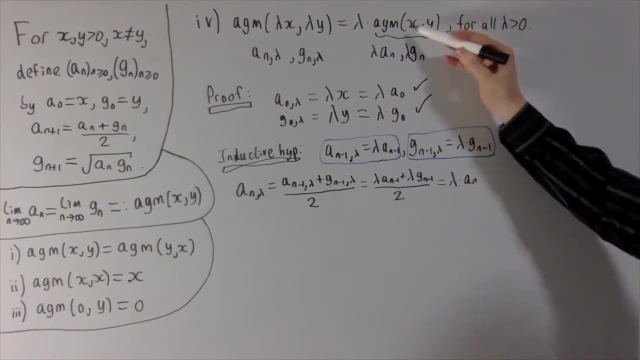 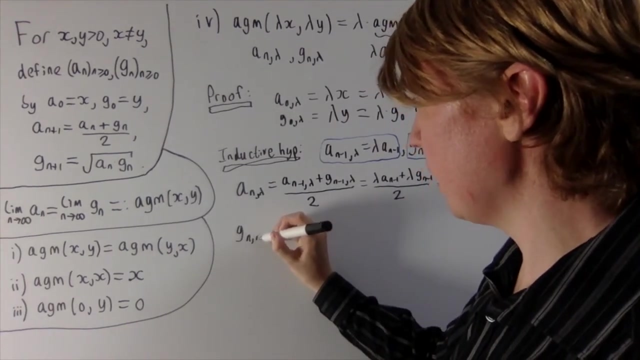 And remembering your definition of what is your an. this is equal to lambda multiplied by an, where now this an is for this sequence without the lambda, And then we can do a similar calculation here for gn- lambda, So the nth term in the g sequence. 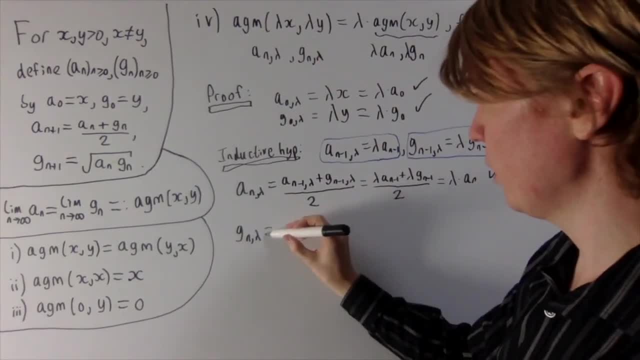 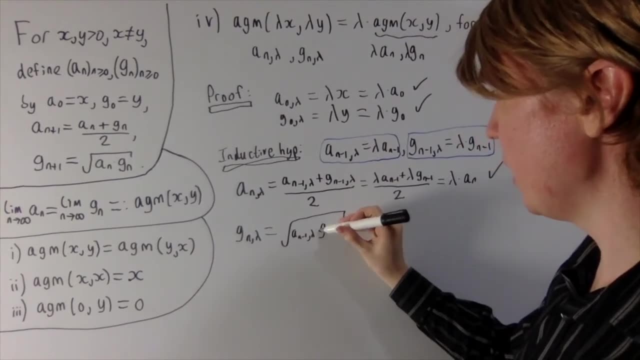 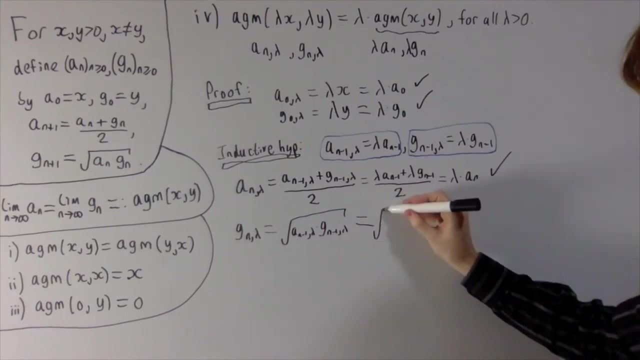 where we started with lambda x and lambda y. So this is going to be the square root of an minus one lambda multiplied by gm minus one lambda. But then we know from the inductive hypothesis we can write this as the square root of lambda an minus one.